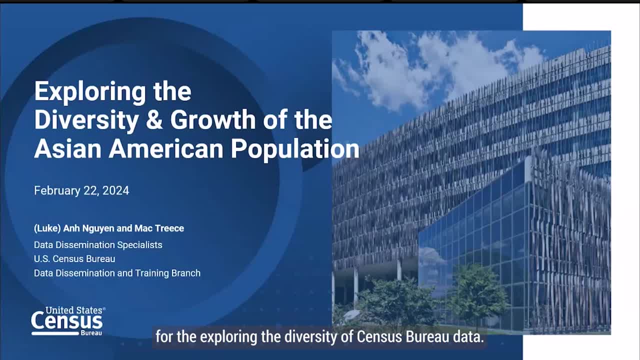 I want to thank you for joining us today for the Exploring the Diversity of Census Bureau Data webinar series. This new series, created by the Census Academy team here at the Census Bureau, is meant to assist the novice to intermediate data user. These webinars are a great opportunity for you to learn from our experts about how to access the Census Bureau data tools and resources. If you wish to follow along, take a moment now to open an additional browser. 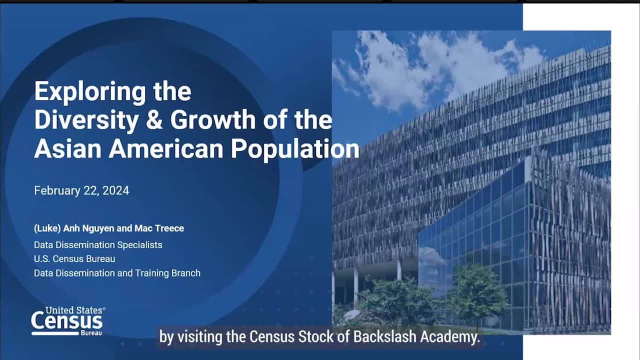 You can register for any of the webinars by visiting censusgov backslash academy. Before I introduce today's speakers, let's go over a few important housekeeping rules. As mentioned earlier, this webinar is being recorded For your convenience. it will be uploaded to our Census Academy site with all supplemental materials relating to the webinar within 30 business days. 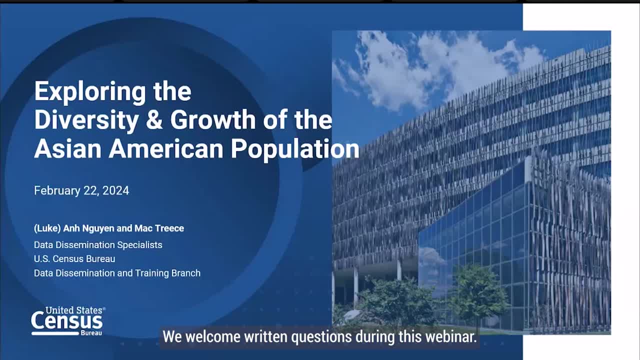 We welcome written questions during the webinar. Please submit your written questions using the QA panel, which is at the bottom center or the right side of your Webex screen. Please take a moment to locate that now. Once you've found the QA panel, make sure you choose all of the questions in the QA panel. 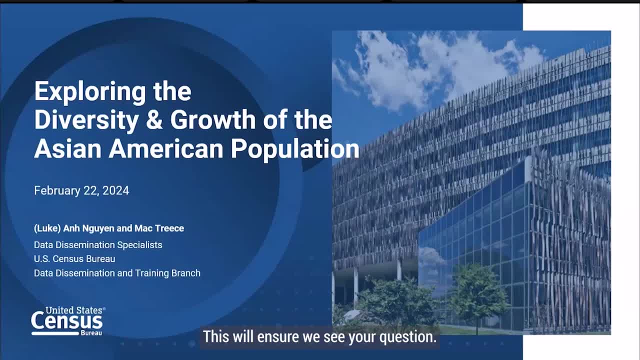 We will be sending out a QA panel to all panelists from the drop down menu. This will ensure we see your question. Also, we ask that you do not include any personal or business identifiable information with your questions. We suggest keeping the chat panel open, as we will provide key links and other resources throughout the webinar. 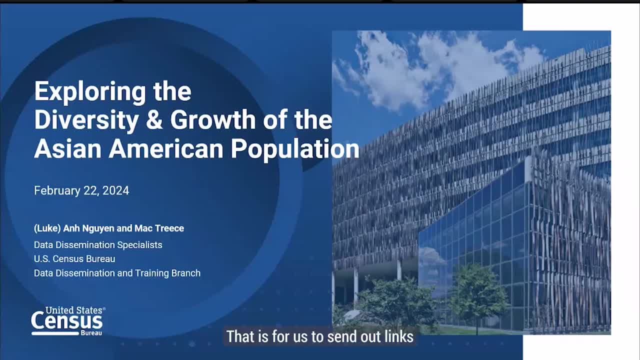 Keep in mind you won't be able to respond to the chat. That is for us to send out links and other resources related to that presentation. My colleagues Kelly Karras and Jolie Golden will be monitoring the QA panel. As time allows, we will answer your question directly through the QA panel or we will share your question with the presenter to respond to during the webinar. 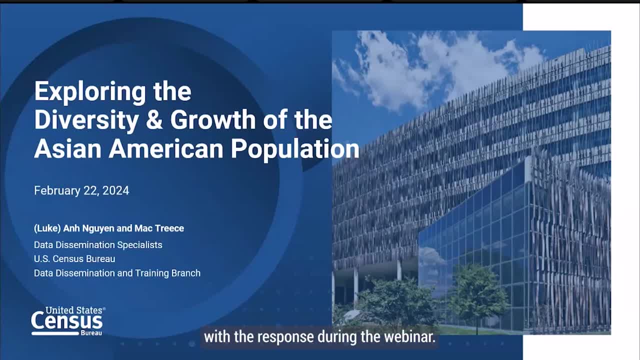 We do not get to all of the questions with the response during the webinar. We will post the questions and responses with the webinar materials on the censusgov backslash academy site within 30 days. As you know, we are in a virtual environment and sometimes technical difficulties might occur. 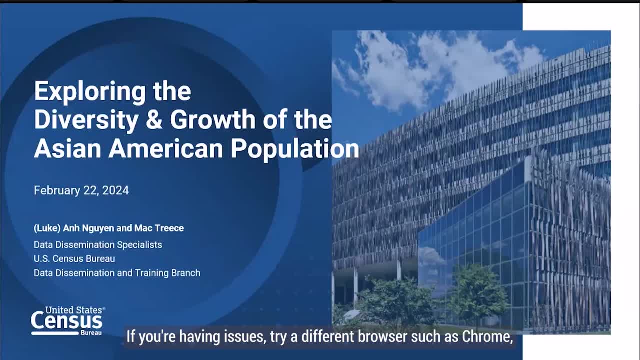 If you are having issues, try a different browser, such as Chrome, or consider logging out and coming back into the session. If you are having audio issues, try selecting the computer audio or calling into the webinar via phone. Now I would like to introduce our speakers Ann Nguyen and Mac Treese. 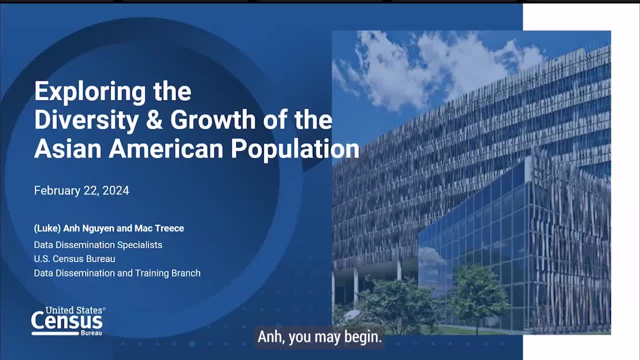 Thanks again for being here today, Ann. you may begin. Thank you, Good morning, Good afternoon everyone. My name is Ann Nguyen and you can call me Luke, It's perfectly fine. I am a data dissemination specialist here at the US Census Bureau since 2008.. 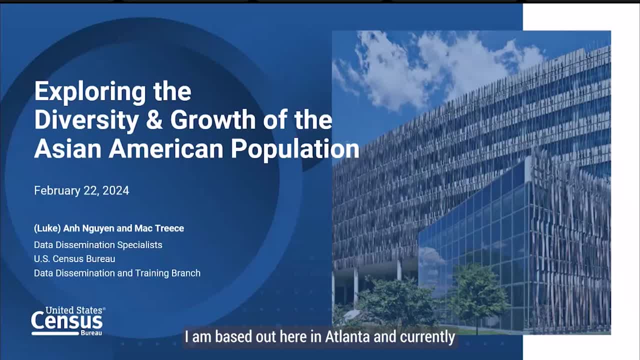 I am based out here in Atlanta and currently I cover the state of Alabama, Georgia and Louisiana, And I have occasionally worked with some of the AAPI national organizations across the country as well, And I can tell you that I have recognized some of you here who I worked with in the past, especially on the past 2020 census, and I really appreciate some of you who have called and shared with me some of your questions prior to this webinar. 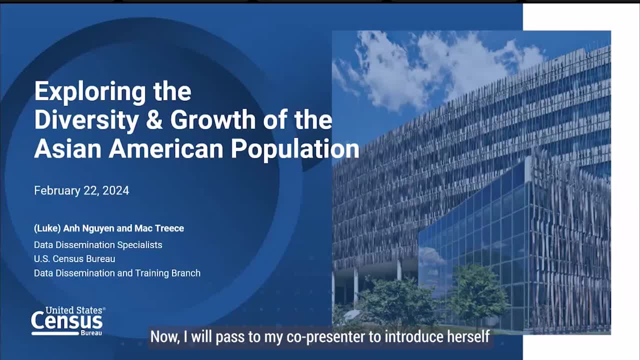 And thank you for joining us today. Now I will pass to my co-presenter to introduce herself. Thanks so much, Ann. My name is Mac Treese and I'm also a data dissemination specialist serving the areas of Northern California and the state of Idaho. 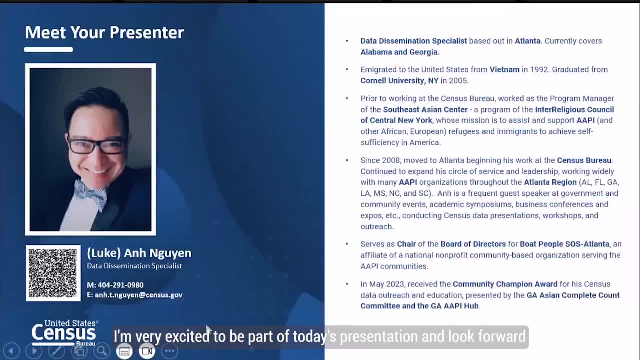 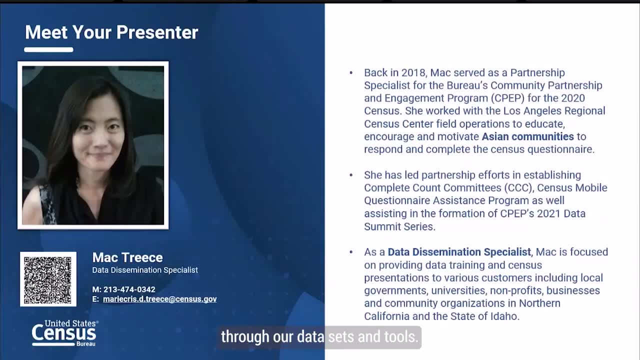 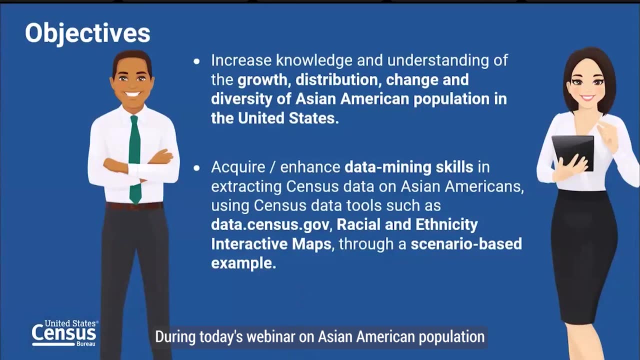 I'm very excited to be part of today's presentation And look forward to sharing data insights into the Asian American population through our data sets and tools Back to you, Ann. Thank you, Mac. During today's webinar on Asian American population in the United States, we would like to focus on number one: increasing our 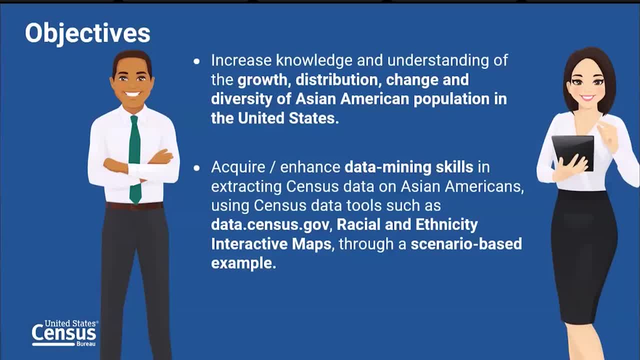 understanding of the growth, the distribution, the change and the diversity of the Asian population by exploring the many surveys, programs and data tools from the US Census Bureau. And, more importantly, we want you to acquire some data mining skills in extracting. 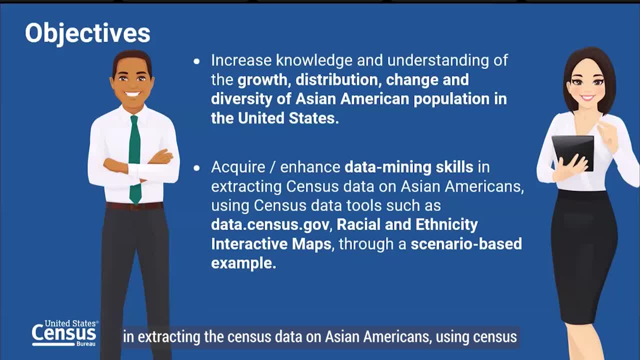 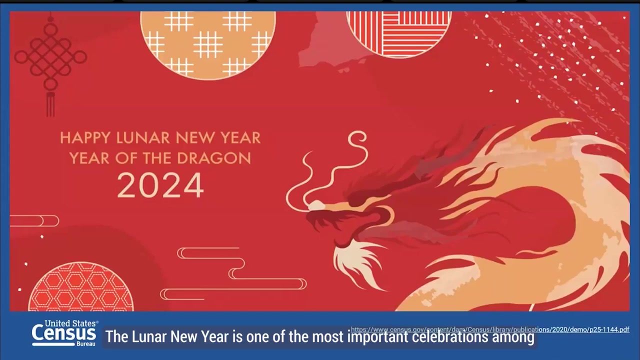 census data on Asian Americans using census data tools such as datacensusgov, racial ethnicity interactive applications and through a scenario-based example. But first, happy Lunar New Year 2024.. The Lunar New Year is one of the most important celebrations among East and Southeast Asians. 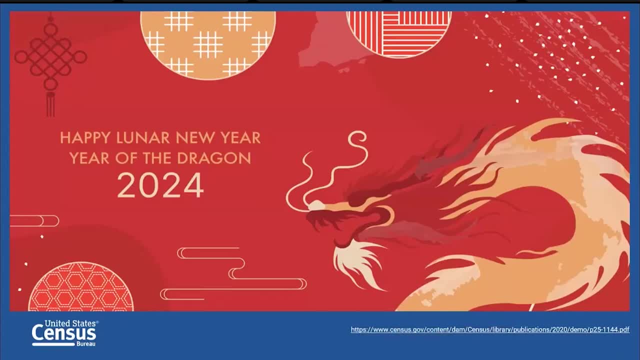 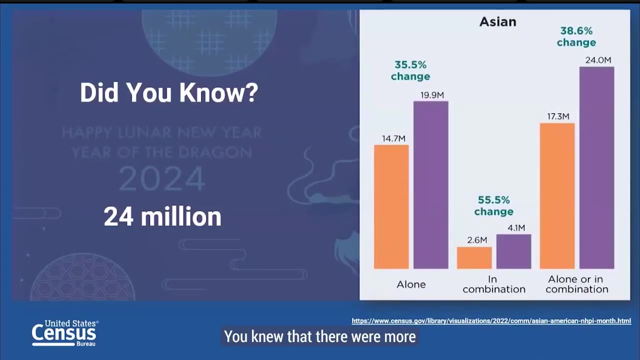 The Lunar New Year is a year of celebration of Asian cultures, including Chinese, Vietnamese, Koreans communities. Now, this year, 2024, Lunar New Year began on February 10th. Did you know that there were more than 24 Asian Americans in the United States, according to the 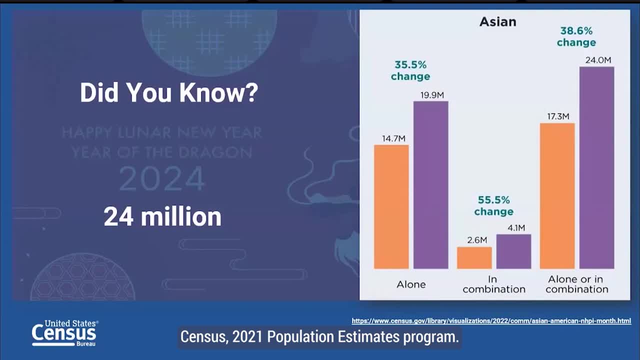 US Census 2021 Population Estimates Program So we can do some work on the encyclopedic. so you can find all the resources you need in the link that will be in the description. The Lunar New Year dicertificates include all the resources that will be provided by: 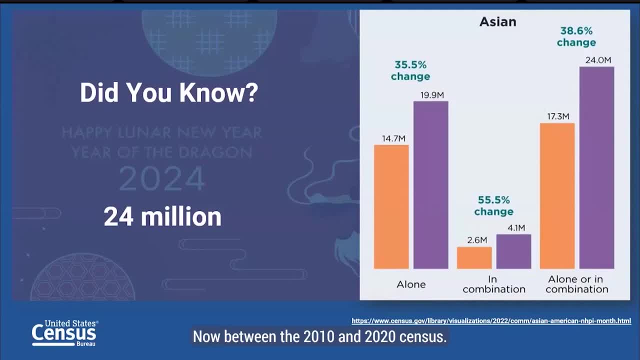 the US Census Bureau, while connecting Asian Asian Americans to the global community. The Lunar New Year 5-year ceremony will be celebrated on May 5th 2021 – a time when more than 1,000 Asian Americans will be able to join the group. 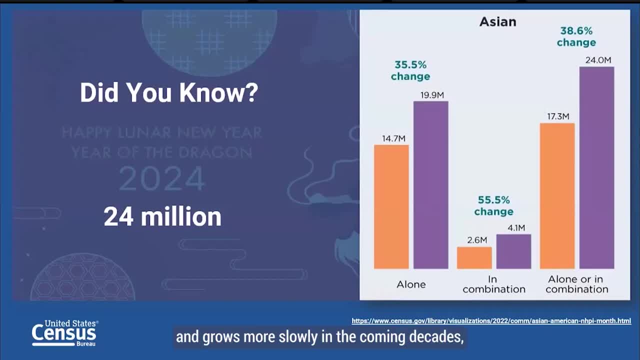 In addition to the five-year celebration of the Lunar New Year, we will also sinsong a More slowly. in the coming decades, the United States is projected to continue to become more racially diverse. The fattest growing racial or ethnic group in the United States is people who 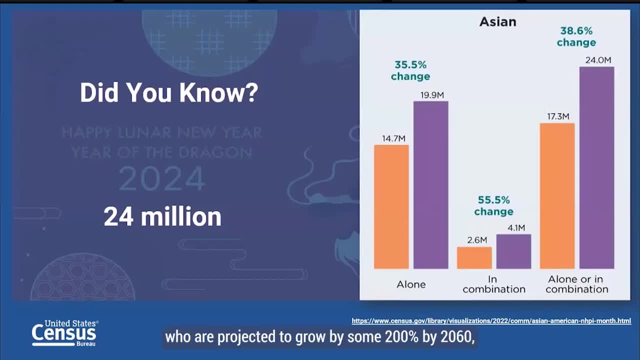 are two or more races who are projected to grow by some 200 percent by 2060, largely by the result of high rates of natural increase. Now the next fattest is the Asian population, which is projected to double by 2060.. For the Asian population, 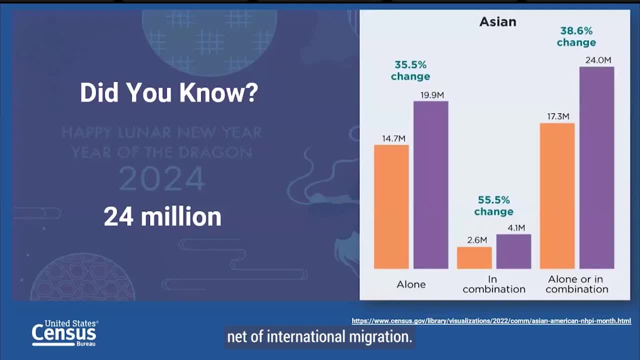 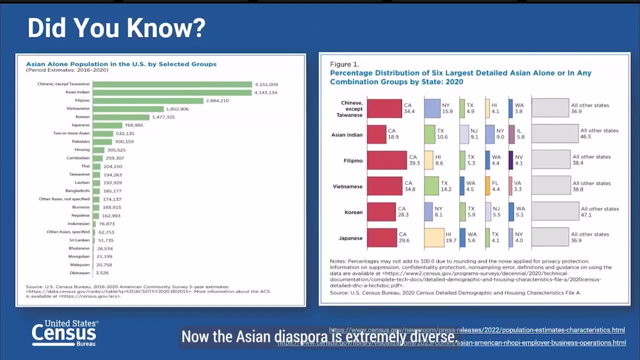 the driving force behind the growth is high net of international migration. Now the Asian diaspora is extremely diverse. For example, using the Latin American diaspora, the Asian diaspora is extremely diverse. Mass suceder is a roastitten background with a USDA. based on survey data from. 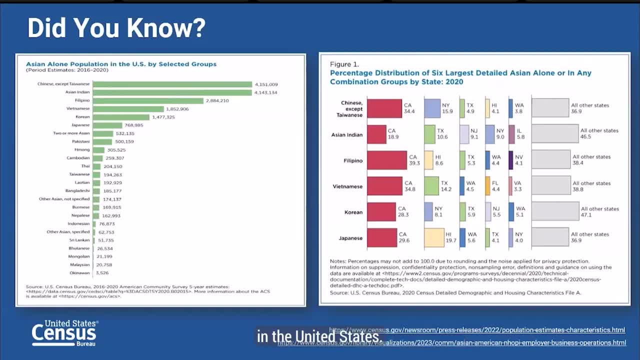 the 2016 and 2025 year American Commuter Survey. The Census Bureau publish data for 21 detailed groups in the United States under the umbrella of Asian alone, including 4.2 million people reporting Chinese, excluding Taiwanese, and 3,526 people reporting. 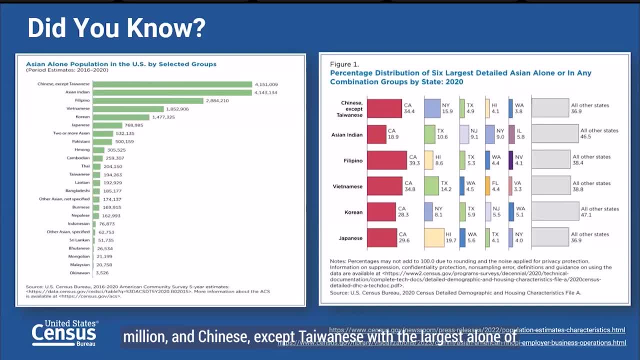 was the largest alone group- 4.4 million- and Chinese, except Taiwanese, was the largest alone or in any combination group by 5.2 million, Now followed by Filipino, 4.4 million, Vietnamese, 2.3 million, Korean, 2 million Japanese. 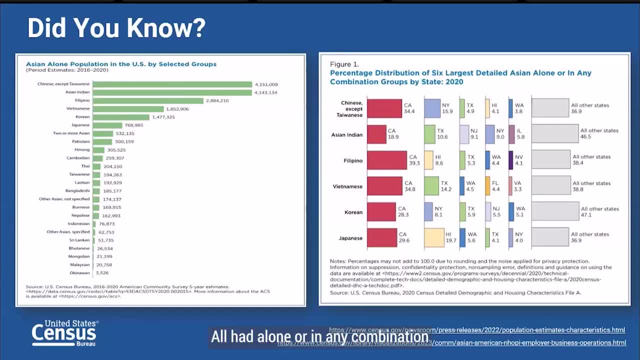 1.6 million. all had, alone or in any combination, population over 1 million in 2020.. The state of California had the largest Asian population, with 7.1 million, followed by New York a bit over 2 million, and Texas, close to 2 million, at 1.8 million respectively. 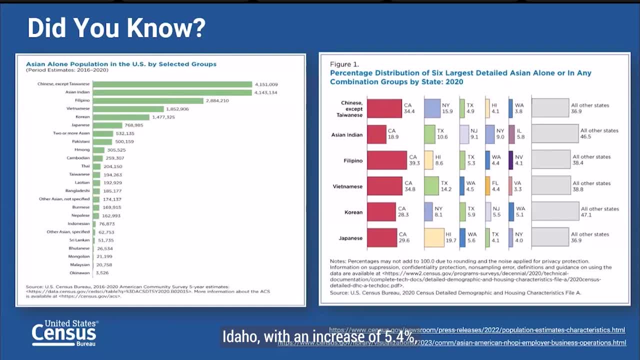 Idaho, With an increase of 5.4%, had the fastest-growing Asian population in 2021.. Among the metropolitan areas, the New York, Newark, New Jersey City metro area had the largest Asian population, followed by Dallas, Fort Worth, Arlington, Texas. 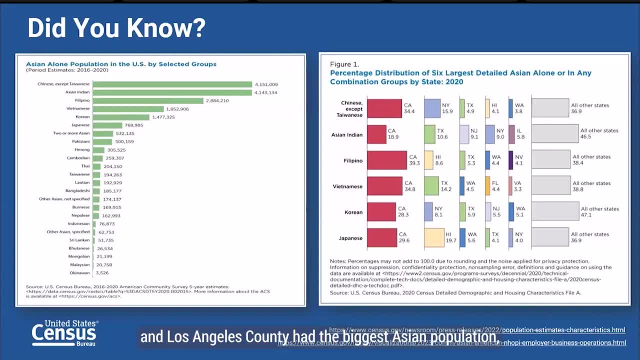 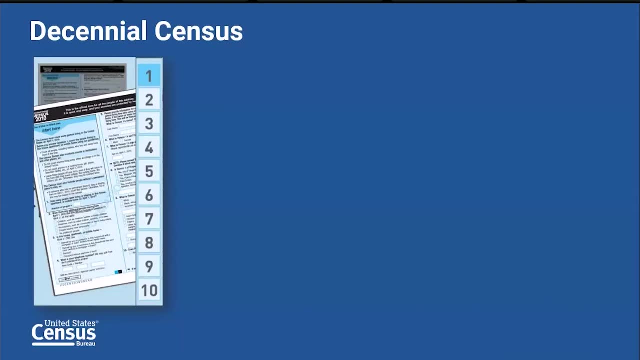 And Los Angeles County had the biggest Asian population, followed by Santa Clara, California and Orange County, all in California. We got the number because based on the decennial census, because every year the US Census Bureau will conduct a census to determine the number of people living in the United. 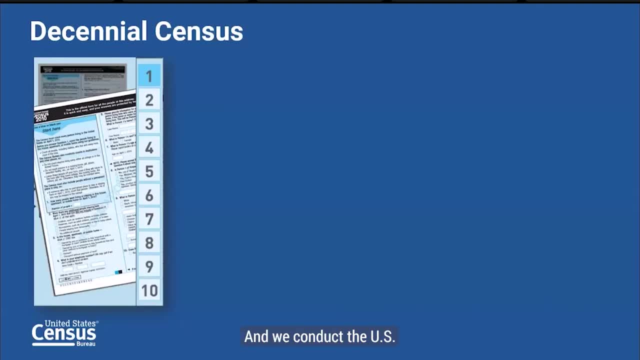 States And we conduct the decennial census in the years ending in zero And the census is the census year. The census year is the year of the census. The census year is the year of the census. April 1st is now considered as Census Day. 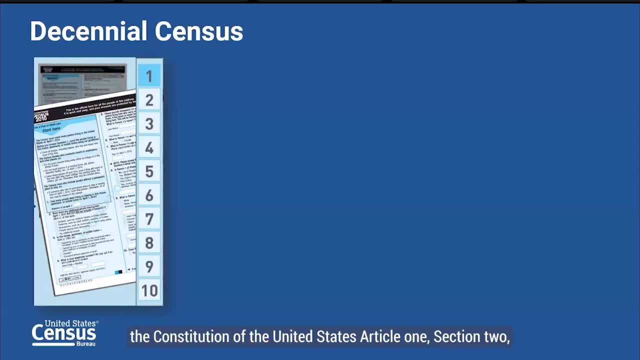 Now, as some of you might know, the Constitution of the United States, Article I, Section 2,, as the census check, the census of population and housing. the census ask question of people in homes and group living situation, including how many people stay in each home and the 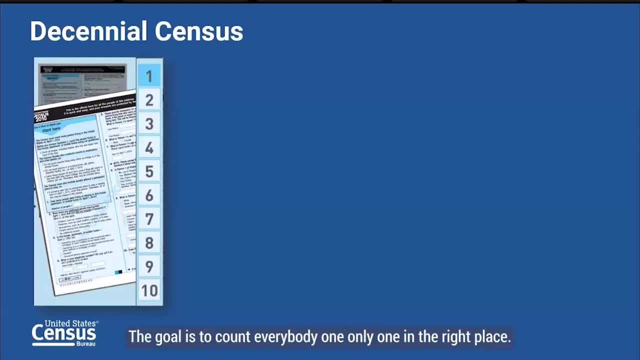 sex, age, race of each person. The goal is to count everybody, one, only one, and in the right place. The data collected by the decennial census are used for apportionment, meaning for dividing among the 400 congressional seats in the House of Representatives. 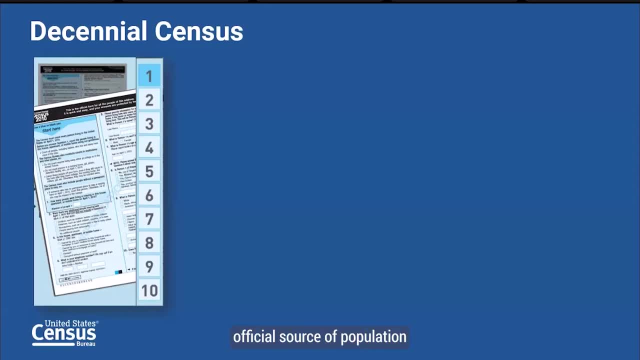 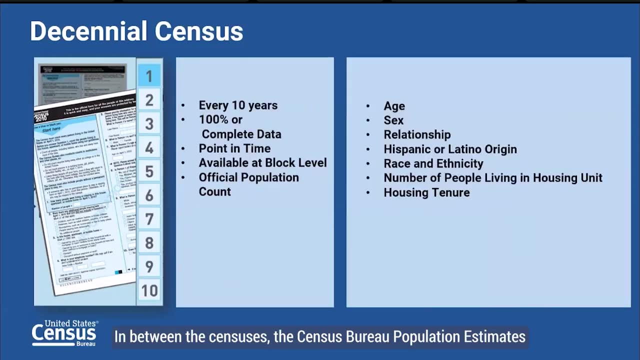 The decennial census is the official source of populations total for April 1st of its decennial year. In between the censuses, the Census Bureau population estimation program produced and disseminates the official estimate of the population for the nation, state, counties, cities and towns. an estimate of housing units for state and counties. 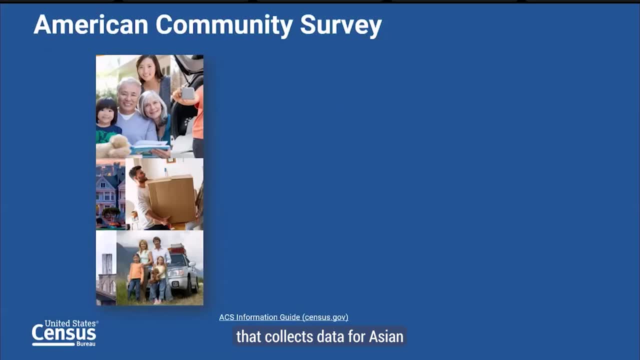 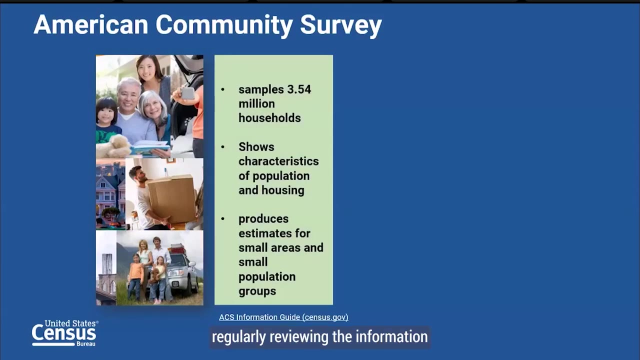 Another important survey that collects data on Asians is called the American Community Survey, which is an annual demographic survey. This is an annual demographic survey program collected by the US Census Bureau. It regularly collects information previously contained in the long form of the decennial. 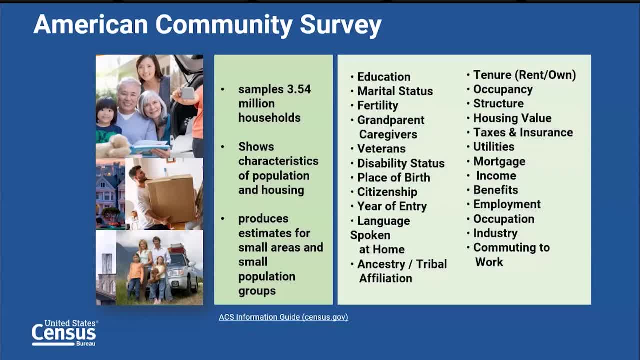 census, including topics such as ancestry, citizenship, educational attainment, income, language proficiency, migration, disability, employment and housing characteristics. Now the one-year estimate. The one-year estimates are available for areas with populations of at least 65,000 people. 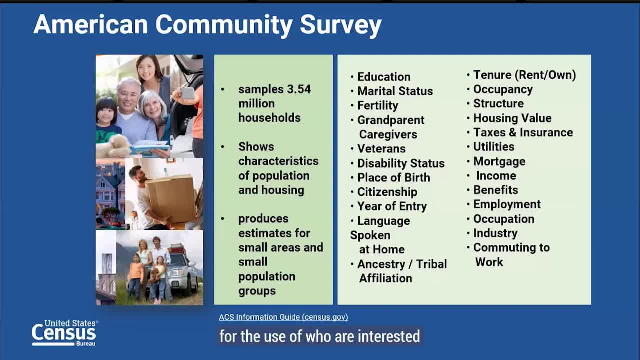 or more. This is most suitable for data users who are interested in short-term changes at the medium to large geographic scales. We also release supplemental estimates that are shown in annual tables summarizing populations for geographies with populations of 20,000 or more. 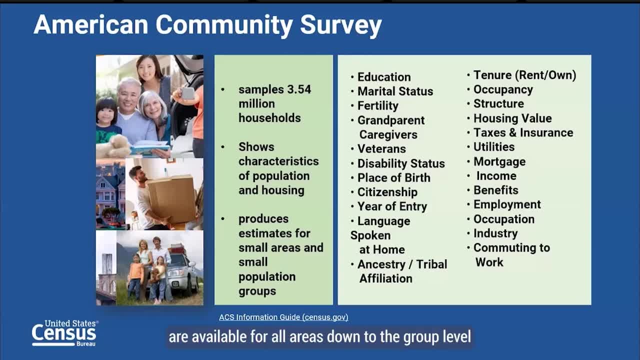 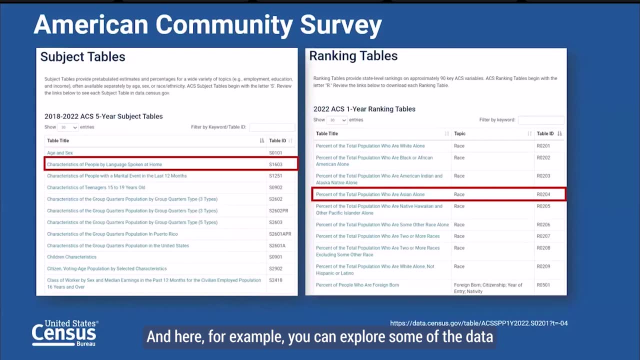 And then the five-year estimate. The five-year estimates are available for all areas, down to the block group level on the order of 600 to 3,000 people, And here, for example, you can explore some of the data on Asian population by, for example: 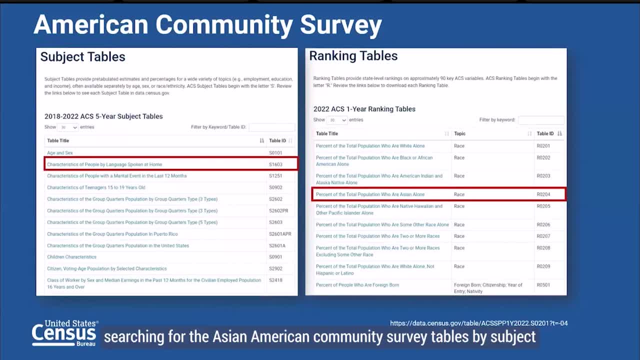 searching for the American Community Survey tables by subject. Subject tables provide pre-tabulated estimates and percentages For a wide variety of topics. ACS subject tables begin with the letter S, for example. So here table S1603, language spoken at home, or table S2902, citizen voting age or table. 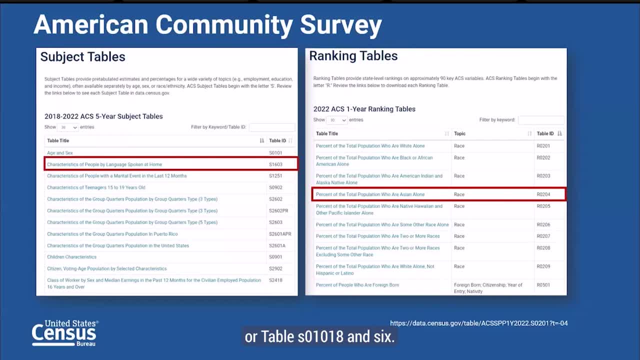 S0101, age and sex, You can learn more about exploring ACS table in-depth. Thank you, And we'll talk about the data that Censusgov in our demonstration later on. We also have ranking tables- provide the state-level rankings on approximately 90 key ACS variables. 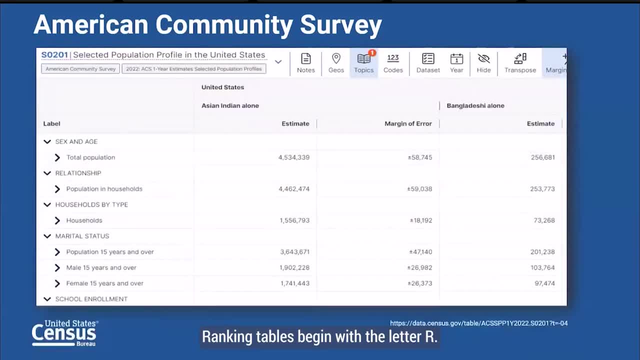 ACS ranking tables begin with the letter R. We can explore data on Asian by look at the data profiles tables. The data profiles table have the most frequently requested social, economic and housing and demographic data. Each of these four subject areas is a separate data profile. 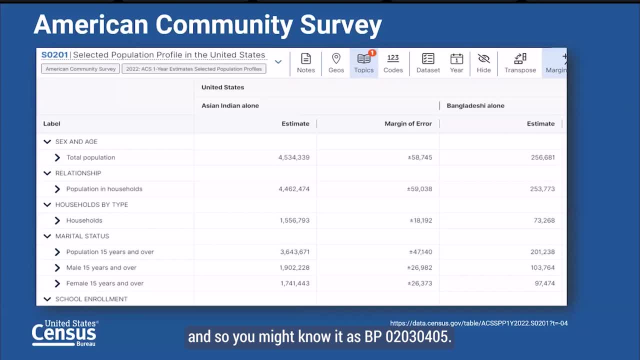 And so you might know it as DP02, DP03, DP04, DP05.. The data profiles summarize the data for single geographic area, most both by numbers and by percentage, And so you might know it as DP02, DP03, DP04, DP05.. 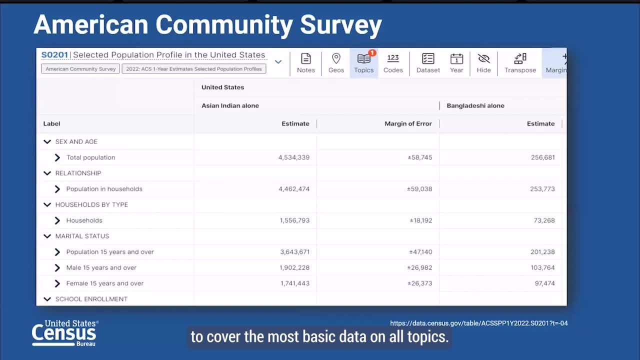 The data profiles summarize the data for single geographical area most, both by numbers and by percentage. They cover the most basic data on all topics, And here an example of what an ACS subject table looks like as I was trying to understand some of the social economic characteristics of the Asian along population broken down. 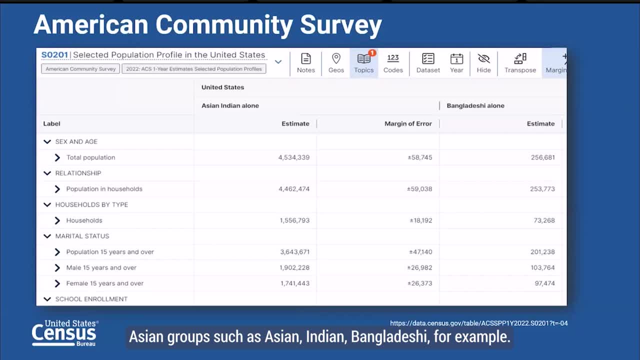 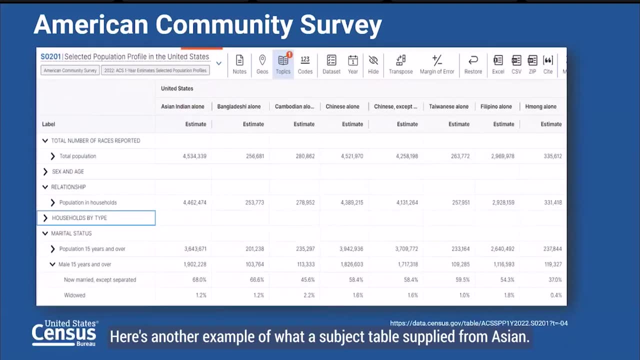 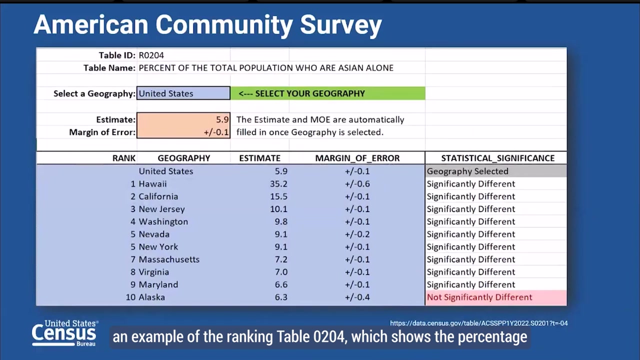 by some smaller sub Asian groups, such as Asian Indian, Bangladeshi, for example. Here's another example of what a subject table would look like on Asians, And here's an example of the ranking table RRI0204,, which shows the percentage of Asian. 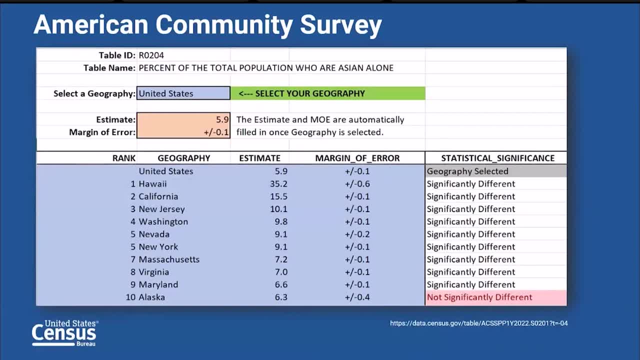 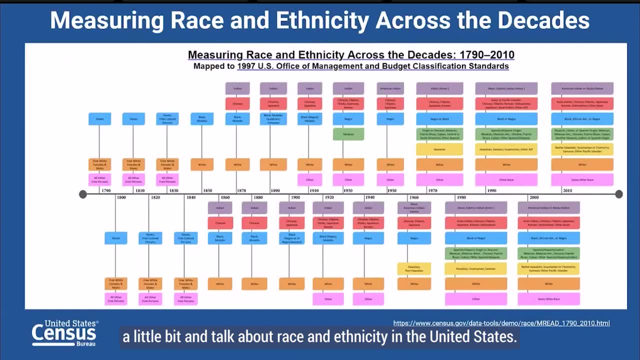 population by state. Now let me switch here a little bit and talk about race and ethnicity in the United States. Now. over the years the US Census Bureau has collected information on race and ethnicity. Now the census form has always reflected changes in society and shifts that have occurred in. 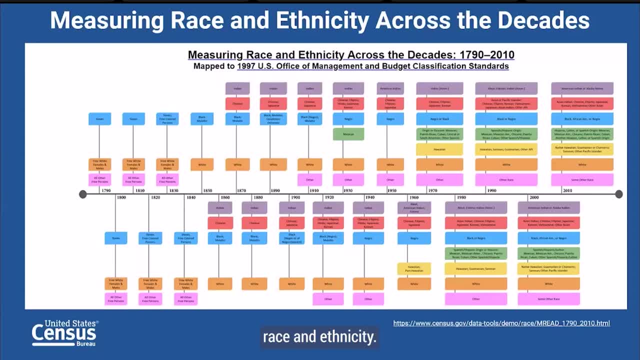 the way the Census Bureau classifies race and ethnicity. Now, historically, the changes have been influenced by shapes, By social, political and economic factors, including emancipation, immigration and civil rights. Today, the Census Bureau collects race and ethnic data according to the US Office of 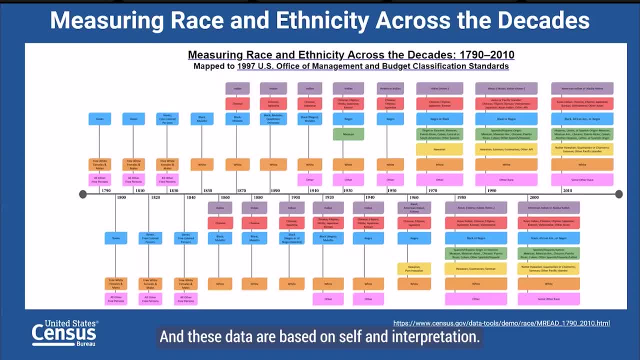 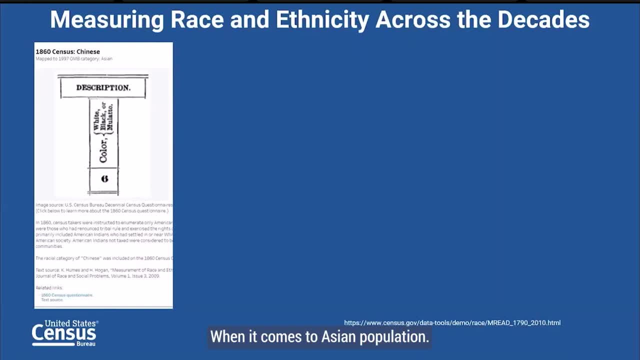 Management and Budget Guidelines, And these data are based on self-identification. Now, when it comes to Asian population, Let me highlight a couple historical moments. For example, in 1860, the racial category for Chinese was included on the 1860 Census. 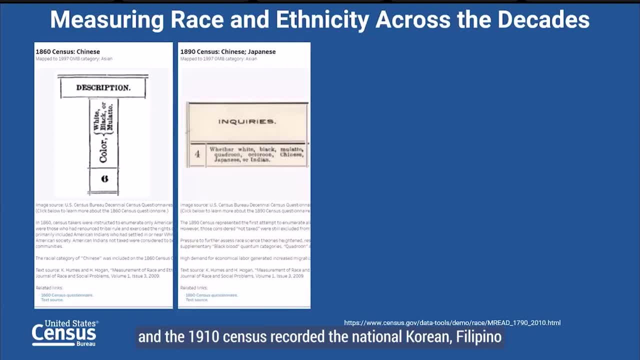 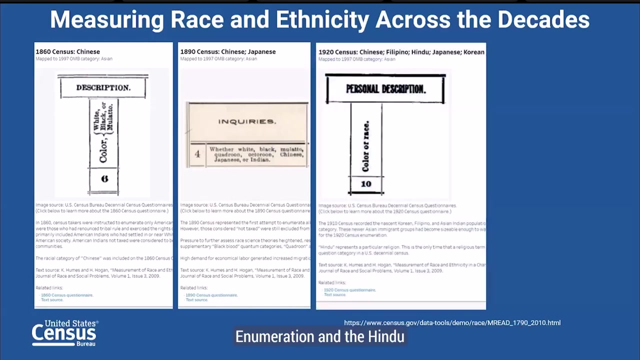 Questionnaire in California only, And then the 1910 Census recorded the national, Korean, Filipino and Asian Indian population as part of the other race category. These newer Asian immigrants Have become sizable enough to warrant creating a separate categories on the 2020 Census enumeration. 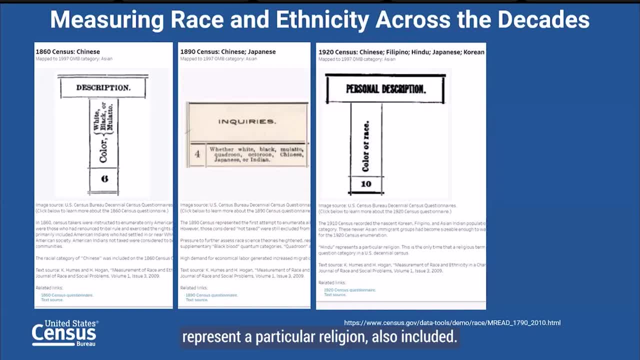 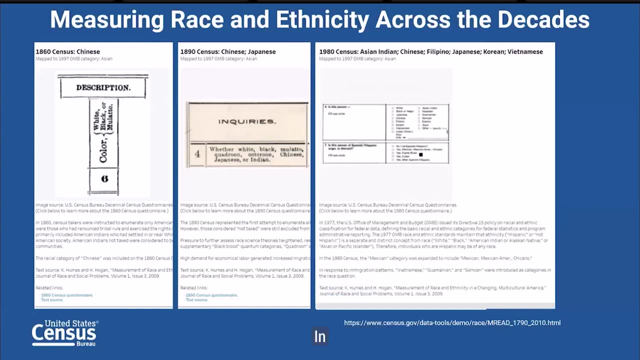 And then Hindu represent a particular religion also included. This is the only time that a religious term has been included as a race question category in the US Decennial Census. In 1977. The US Office of Management and Budget issued a Directive 15 policy on racial and. 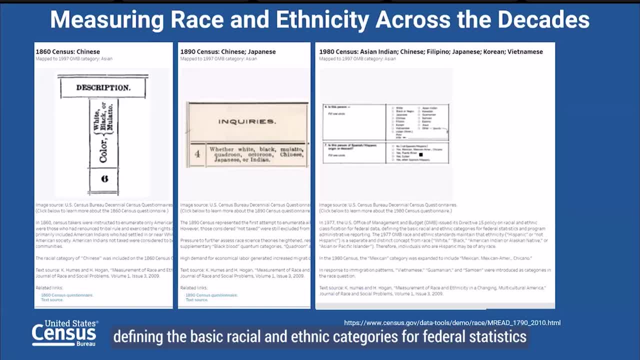 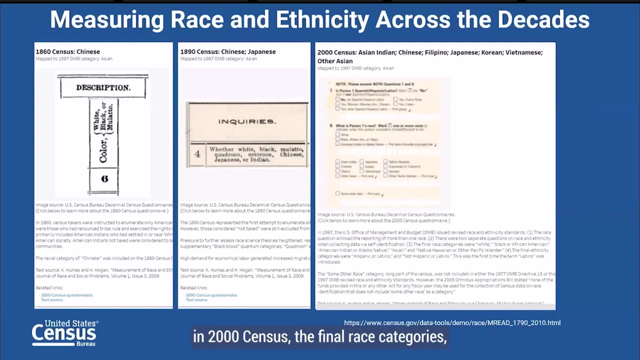 ethnic classification for federal data, Defining the basic racial and ethnic categories for federal statistics and program administrative reporting. So in response to immigration patterns, You can see that Vietnamese, Romanian and Samoan were introduced as categories in the race question In 2000 census. the final race categories were white, black or African American. American. 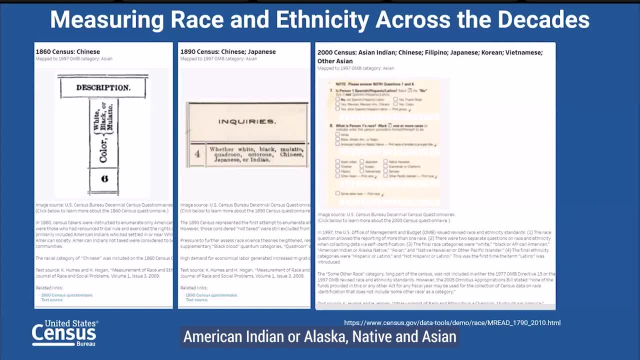 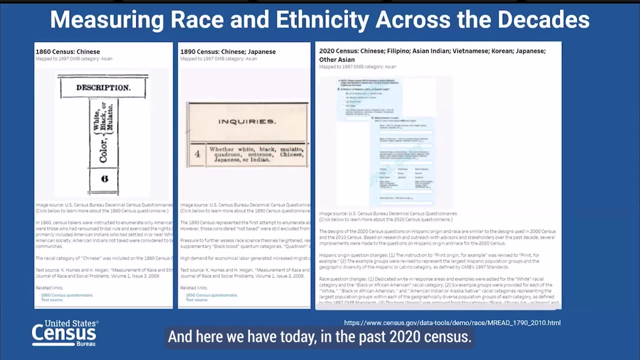 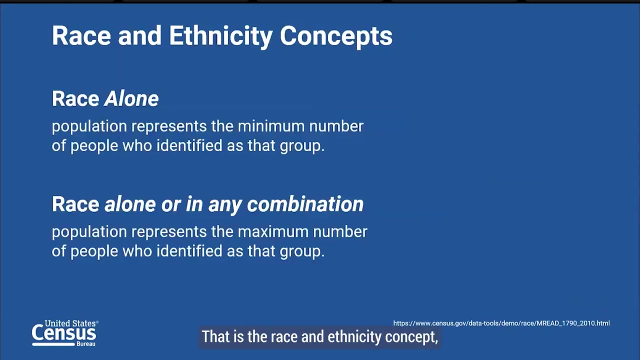 Indian or Alaska Native and Asian and Native Hawaiian or other Pacific Islanders. There were two separate racial categories And here we are today. in the past 2020 census, This is how the Census Bureau has collected data on Asian population To go with, that is, the race and ethnicity concept, because the racial categories included. 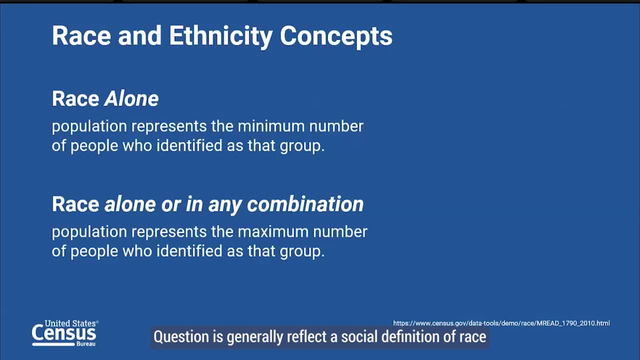 in the census questionnaires generally reflect a social definition of race recognized in this country and not an attempt to define race biologically, anthropologically or genetically. Now, in addition, it is recognized that the categories for race items include racial and national origin or social cultural groups. 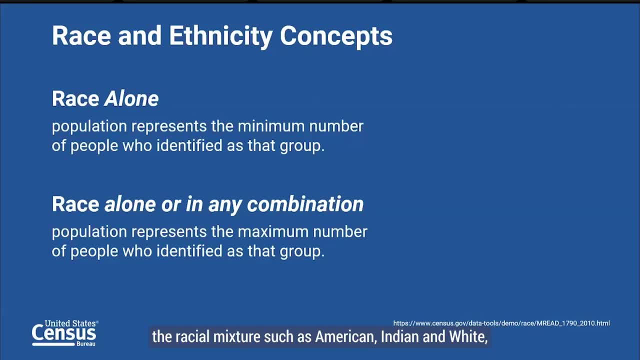 People may choose to report more than one race to indicate the racial mixture, such as American, Indian and white, Asian and white, Asian and black, and people who identify the origin as Hispanic, Latino or South African. This also applies to Hispanic and Asian population with the same national origin. 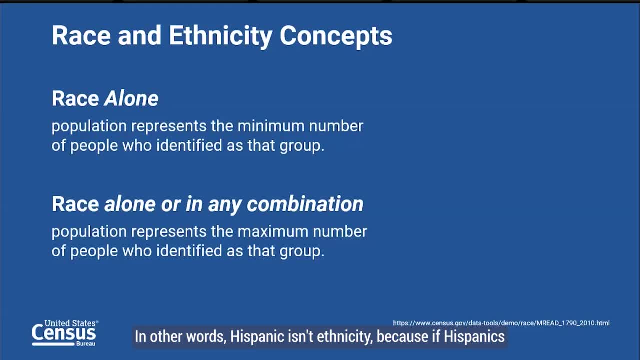 Some groups may have any race. In other words, Hispanic is an ethnicity, because Hispanic can be of any race. But Asian population is a person who having origin in any of the original people of the Far East, the Southeast Asia or the Indian subcontinent, including, for example, India. 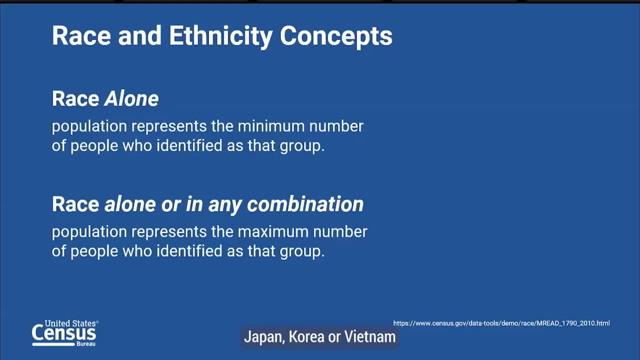 China, the Philippines, Ireland, Japan, Korea or China. In addition, Asian population is considered to be of any race. In addition, Asian population is considered to be of any race. This is because the racial differences are行わ of each national group. 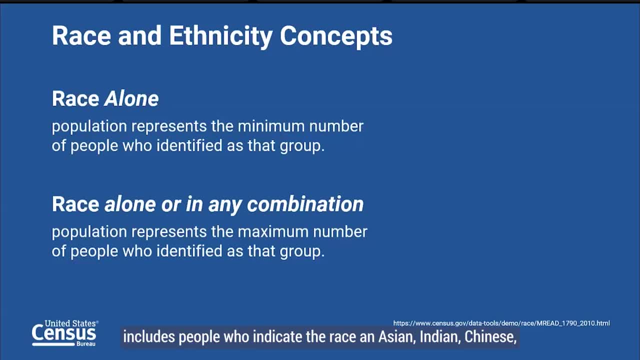 We would like to highlight each population and what they have in common. Korea or Vietnam includes people who indicate the race as Asian, Indian, Chinese, Filipino, Korean, Japanese, Vietnamese and so on. The concept of alone or in any combination also apply only to respond to the race question. 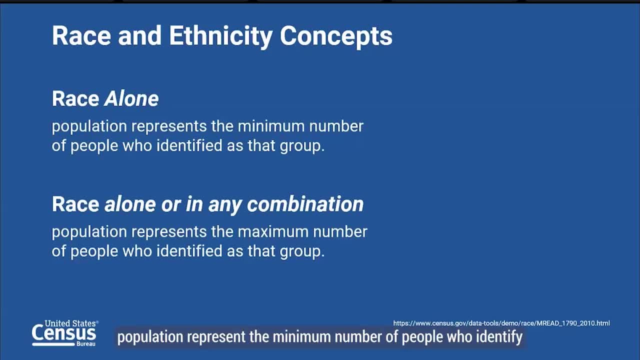 The race alone. population represents the minimum number of people who identify as that group includes those who are reporting only one response, such as only Chinese. As you see in the 2020 Census questionnaire example that I showed earlier, there's a category for Chinese, Vietnamese, Korean. 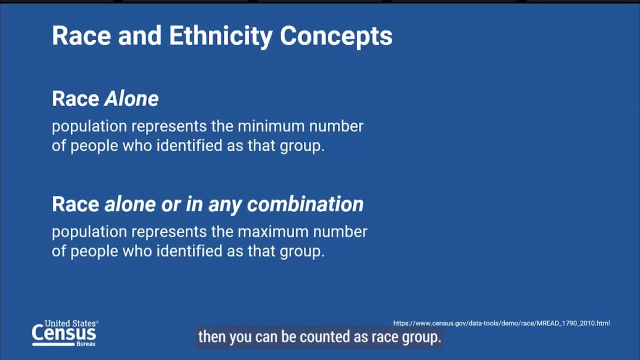 You can check only one response. Then you can be counted as race alone, group, The race alone or in any combination. The race alone population represents the maximum number of people who identify as that group. Now it includes those who reported only one response, such as Chinese, and those who reported 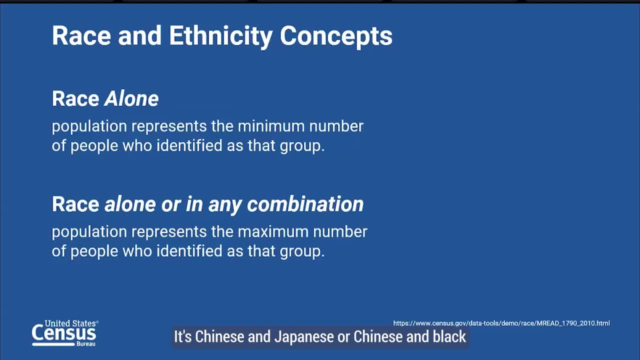 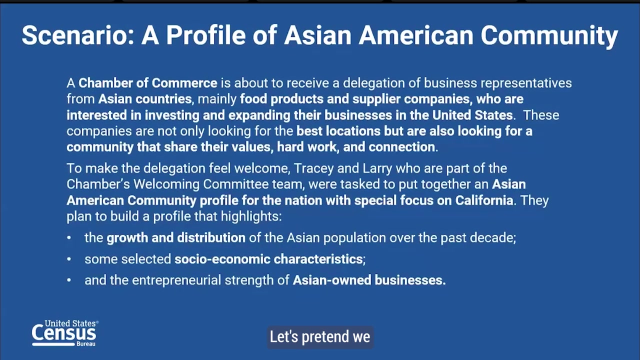 multiple responses, such as Chinese and Japanese or Chinese and Black or African American. So those were the basic overview of some of the key responses. So let's talk about the next slide. So let's talk about the main objectives of this new Initiative. 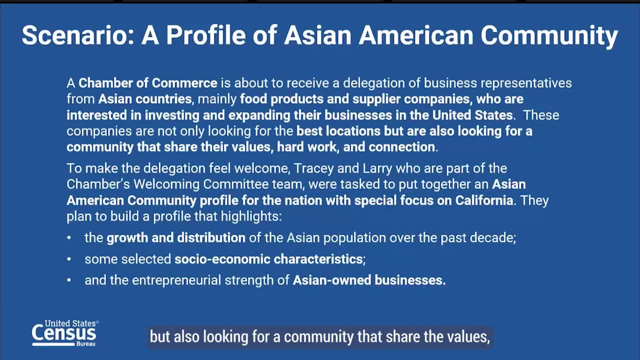 The main objectives are as follows: To look at the deliberative within the Asia-Pacific context, but also looking for a community that share the values, hard work and connection. So to make the delegation feeling at home, Tracy and Larry, our two fictional customers, 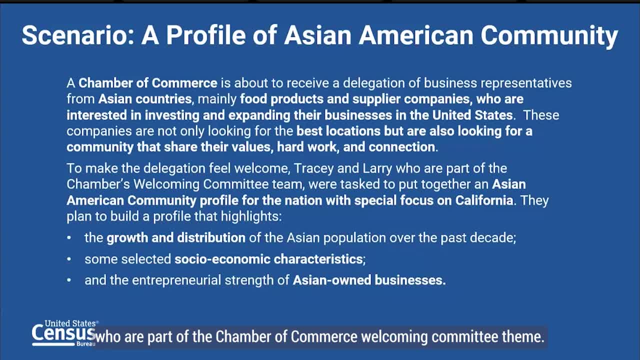 who are part of the JetWeb Commerce welcoming committee team. they were tasked to put together an Asian American community profile for the nation, with special focus on California. So Tracy and Larry then plan to build a profile that highlights number one: the growth and 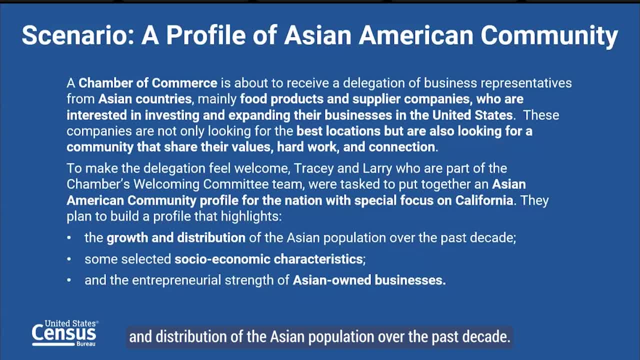 distribution of the Asian population over the past decade. They want to feature some of the selected social and economic characteristics of the Asian population And, more interesting, they want to show the entrepreneurial strength of the Asian-owned businesses. So what does that mean? 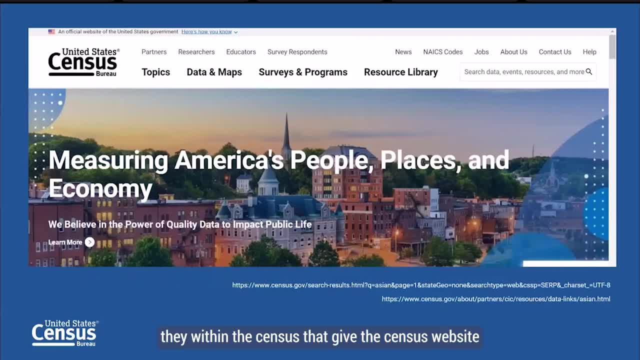 So what the team did first. they would then visit censusgov, the census website, And in the search box- and you can see on the top right corner- and they type in Asian in the hope of looking for finding something, anything that related to Asian. 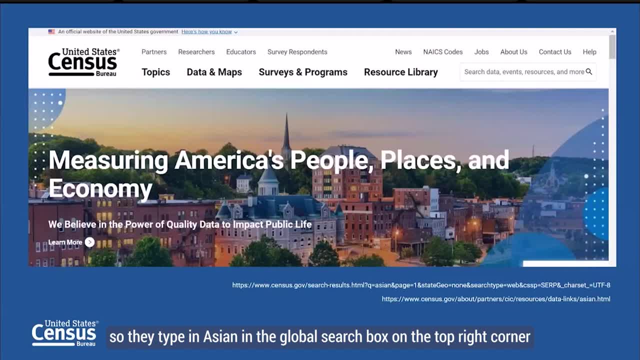 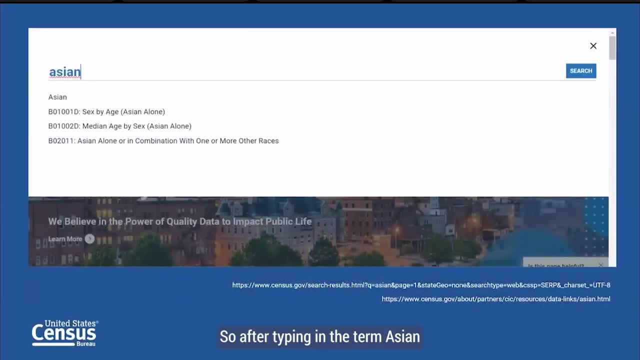 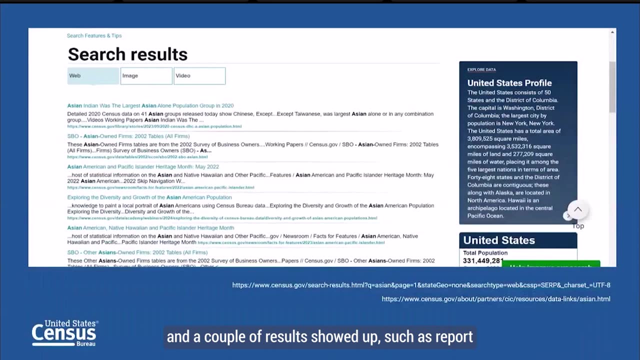 So they type in Asian in the global search box on the top right corner. So they found a couple of good results, such as report. So after typing in the term Asian and a couple of results showed up, such as reports. 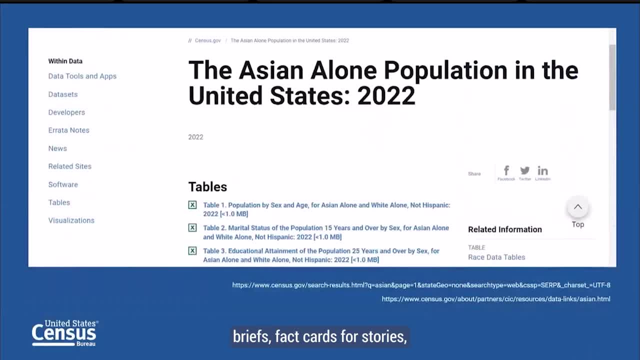 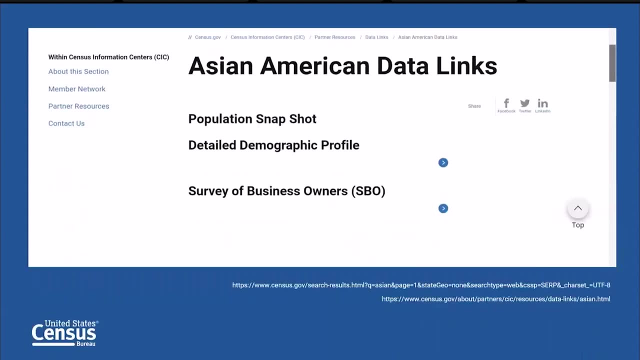 briefs, facts, stats for stories and, most importantly, lots of data tables and an Asian American data link. So this is a good start Now. so I Okay, All right. So after scanning through a few of these results and resources, they also discovered: 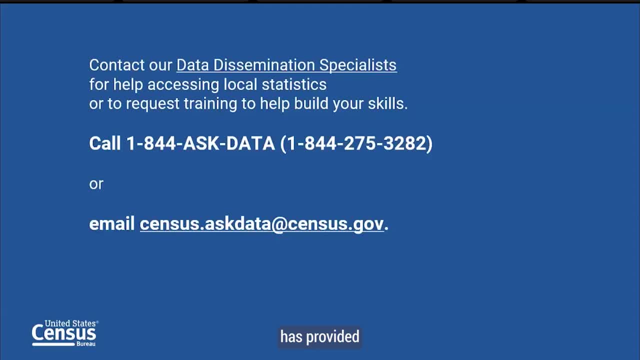 that the Census Bureau has provided a call number, a phone number for them to call to ask for more data. So they went ahead and called 1-844-ASK-DATA or 1-844-275-3282.. So they were transferred to a data dissemination specialist who told them that they were interested. 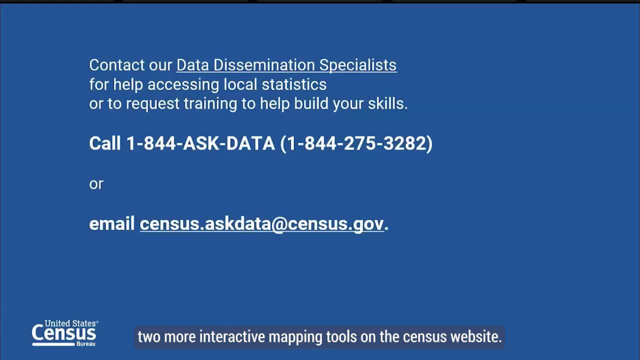 in this and when they went to the census website, who told them to go ahead and explore two more interactive mapping tools on the census website. One is called Race and Ethnicity in the United States: 2010 census and 2020 census. 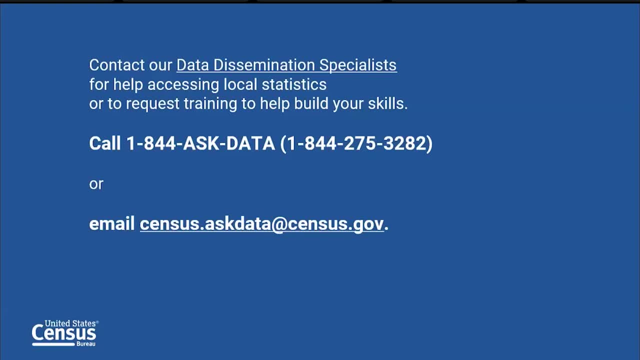 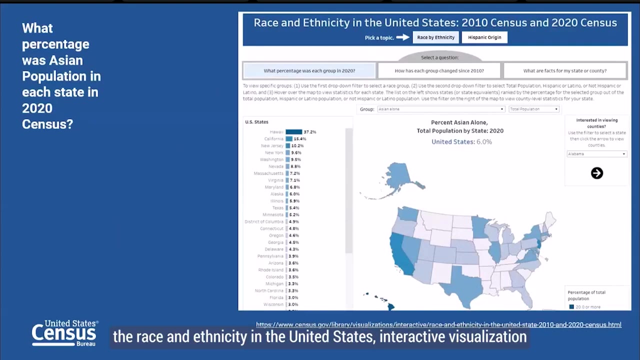 And the other one is called Detailed Races and Ethnicities in the United States and a data search tool called datacensusgov. So let's go ahead and begin exploring these tools, For example, the Race and Ethnicity in the United States. Interactive Visualization Tool. 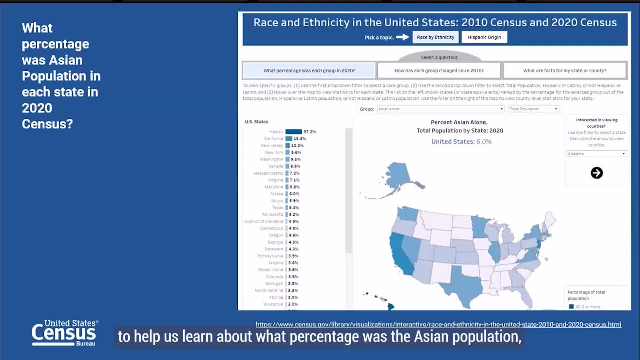 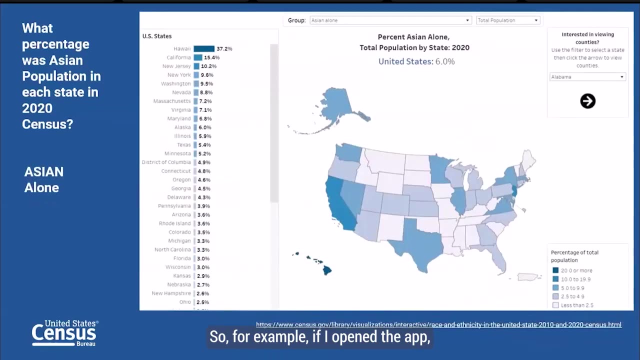 helped us learn about what percentage was the Asian population, how the Asian population has changed since 2010. census by state and by county. For example, if I open the app, the application and then if I select the Asian alone category, the tool would then give me a map which shows the distribution of Asian alone population. 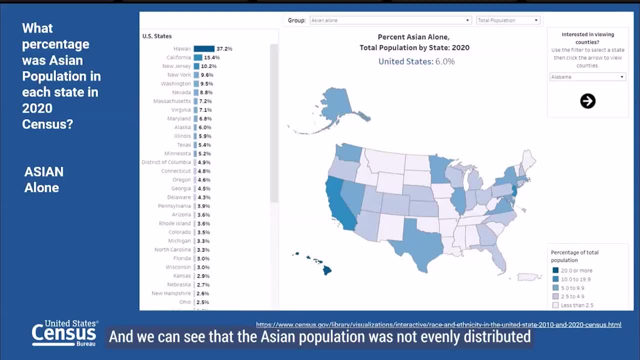 by state And we can see that the Asian population was not evenly distributed across the United States. according to the 2020 census- And you can see the column on the left- only three states- Hawaii, California and New Jersey- had 10% or more of the population who identified as Asian alone. 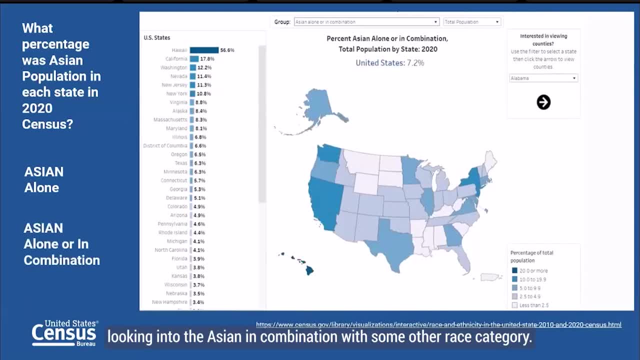 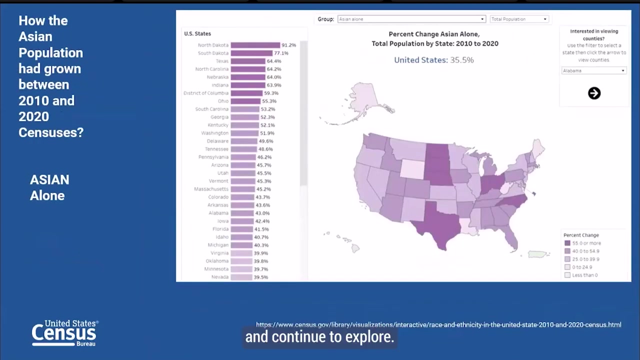 Now if we are looking into the Asian in combination with some other race category, we can see that Hawaii, Washington and Nevada are three states with the highest percentage of the population who identified as Asian in combination with one other race And if you continue to explore, they can learn how to see how the Asian population 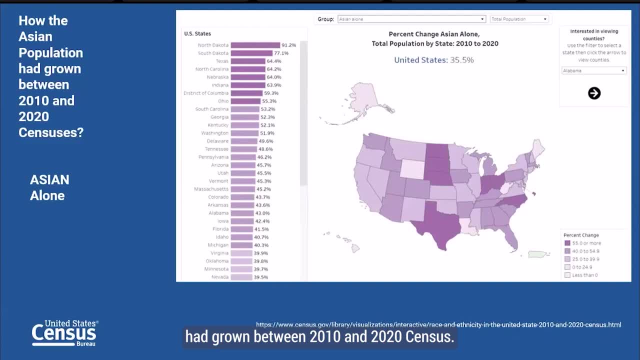 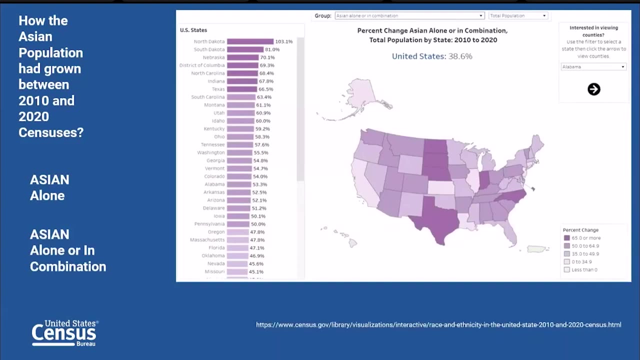 had grown between 2010 and 2020 census And you see the Asian alone category rose by 35.5%. But if you look into the Asian alone or in any combination, the Asian population has grown by 38.6%. Okay, 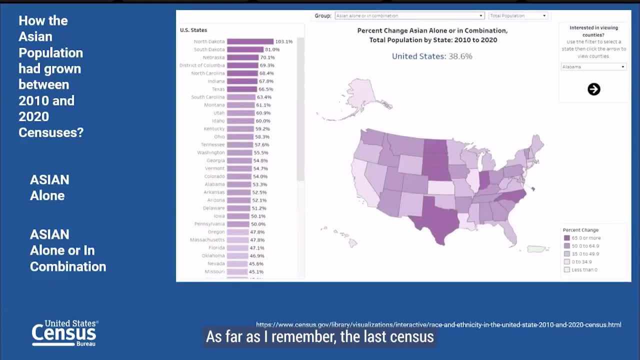 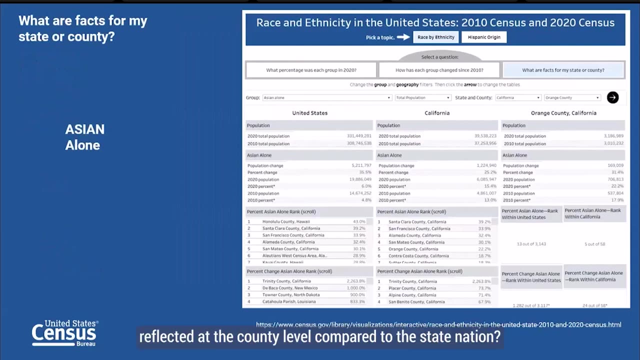 As far as I remember the last census, between 2000 census and 2010 census, the Asian population grew by 46%. Now how did the change in Asian population reflected at the county level compared to the state and nation? So we can go to explore the third feature on the app, for what are the facts for my state? 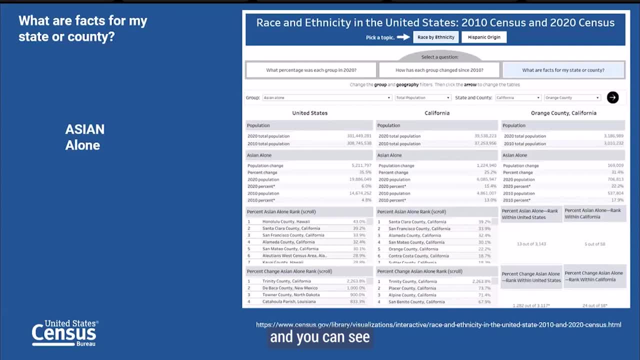 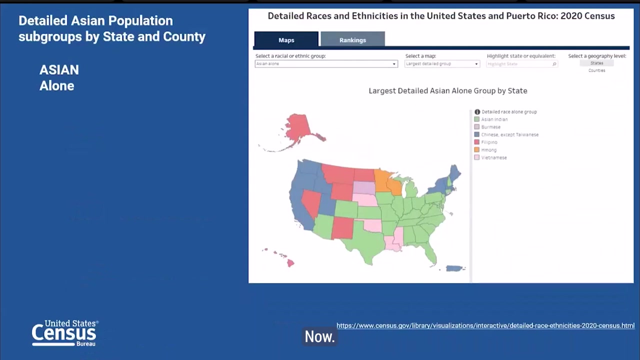 or county, for example, And you can see a lot more facts or data on Asian alone and Asian category, And you can be able to view and compare them at the nation level, the state level and the county level. Now, so being aware of the diversity within the visiting delegation. so the Chamber of 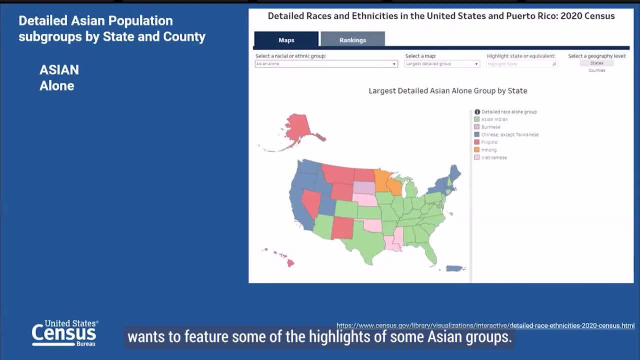 Governors team further wants to feature some of the highlights of some sub-Asian groups. They then explore the mapping and ranking features on the 2020 census detail races and ethnicities interactive mapping tool, which helps them to explore further, to learn more about which state has the high concentration of some selected Asian population subgroups. 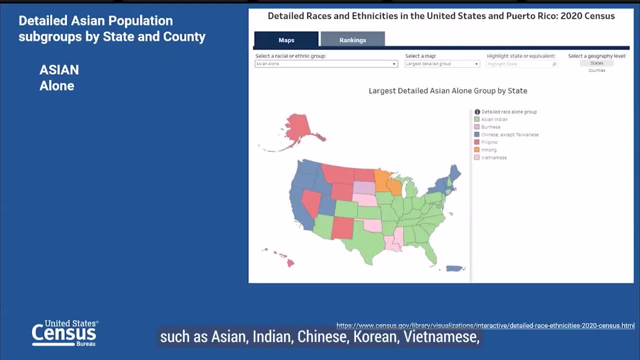 such as Asian Indian, Chinese, Korean, Vietnamese and Asian. Okay, Thank you. Next slide. So we have two main categories of Asian Indian alone and Asian Indian combination categories. One is the Asian Indian alone population And it's the Asian Indian alone population. 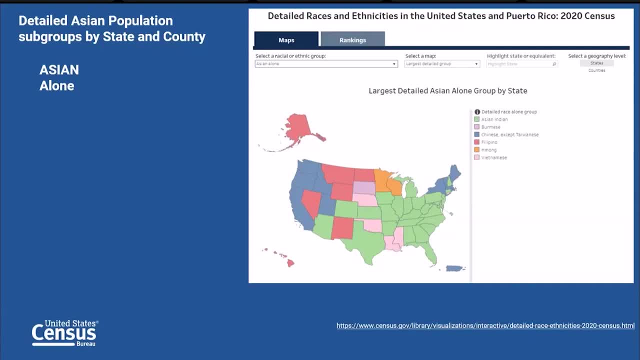 And the second category is the Asian Indian alone population. So Asian Indian alone population has increased by 54.7% to more than 4.3 million between 2010 and 2020 census And they become the most popular Asian alone in the country. 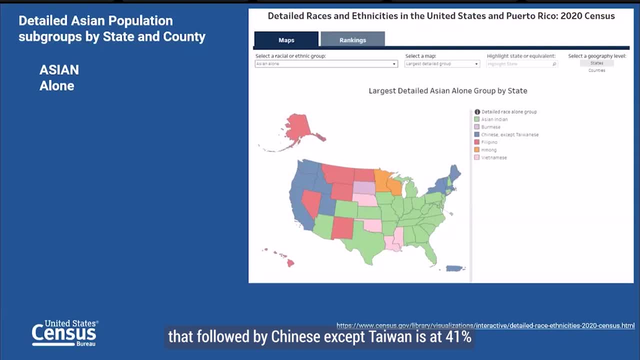 That followed by Chinese, except Taiwanese, at 4.1%, And then the third category is the Asian Indian alone population, And then Filipino alone, 3 million, Vietnamese, close to 2 million, Korean, 1.5 million and Japanese alone at 741,000.. 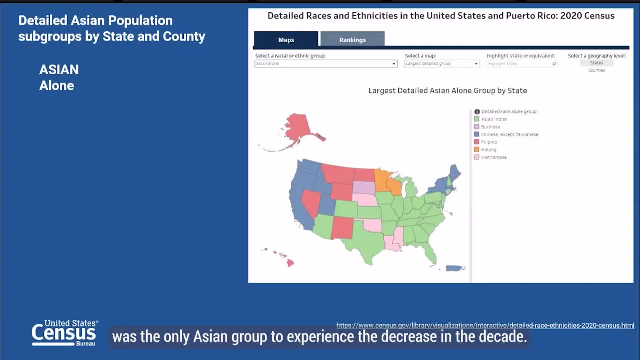 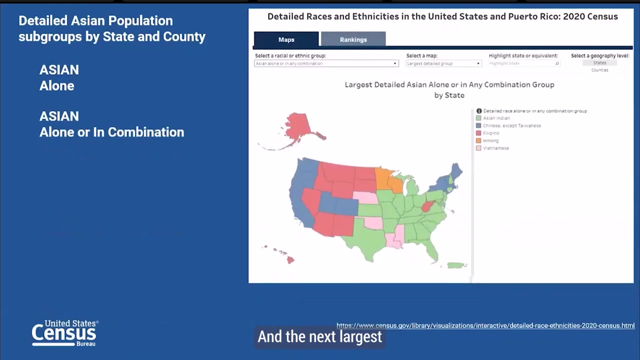 Now the Japanese population and the Laotian alone population were the only detailed Asian groups who experienced a decrease in the decade, And the alone or in combination population increased by 26-by 20.6% and 9.5% respectively, And the next largest Asian alone or in combination groups population that grew from 2010 to 2010. 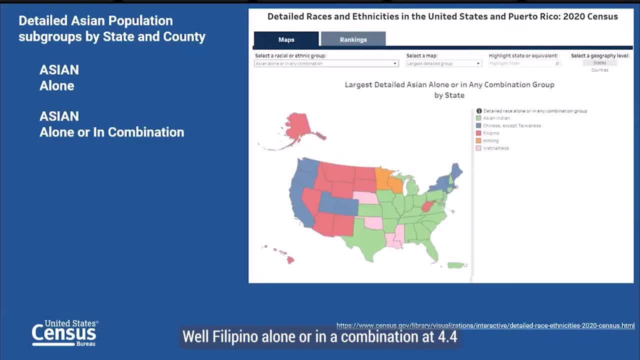 census were Filipino alone or in the combination: The 4.4 million Vietnamese in combination: more than 2.2 million, The Korean more than 2 million And the Japanese alone in combination, more than 1.5 million. And then you can go ahead. 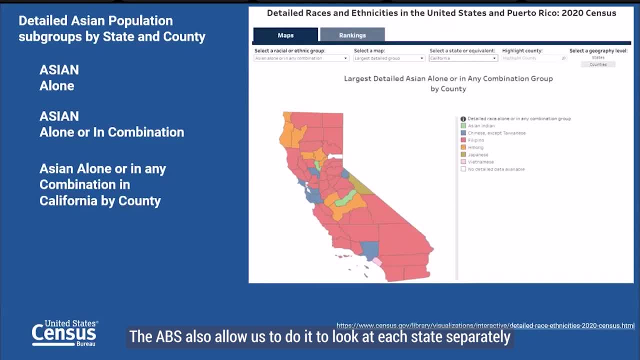 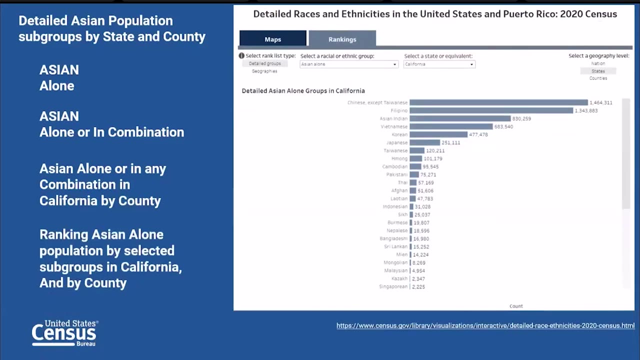 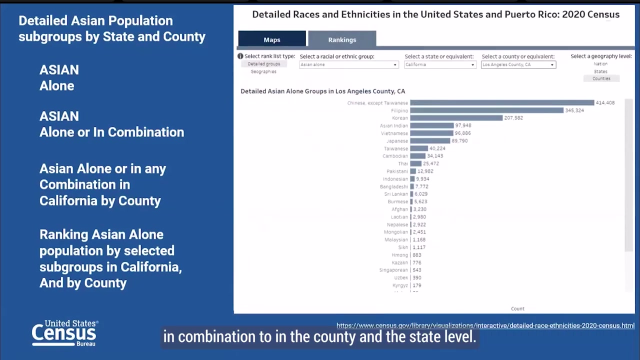 The apps also allow us to drill in, to look at each state separately and to see the distribution of these some selected Asian subgroups per slide, And the rankings feature on this app also help us to understand which is the largest alone group or which is the largest in combination group in the county and the state level. 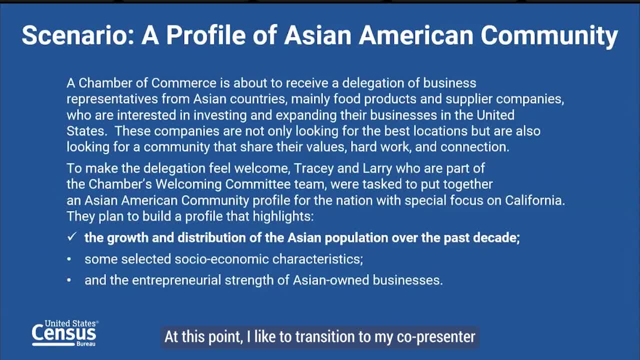 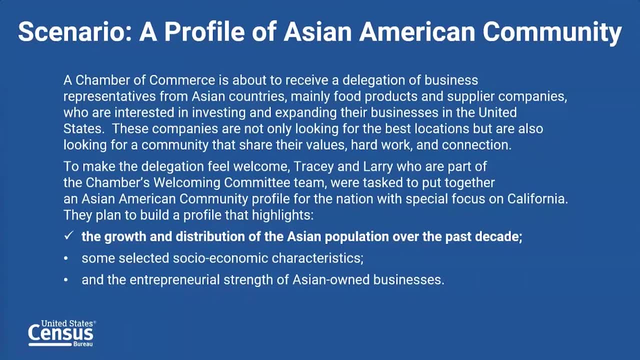 At this point I'd like to transition to my co-presenter, Matt, to continue with the scenario. Thank you so much, Thank you, Thank you. Thank you so much, Anne. So, now that the Chamber team of Tracy and Larry have met the first objective of getting 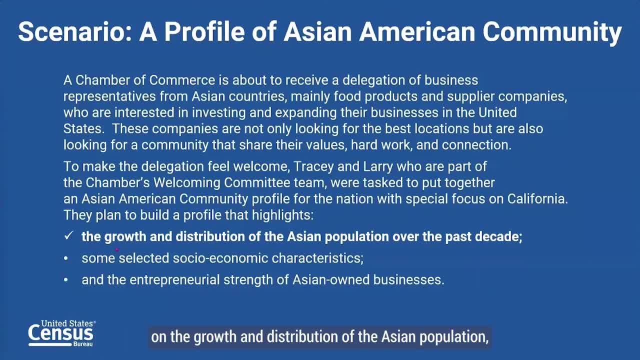 the information on the growth and distribution of the Asian population. it's time to tackle the next two items on their list, So we will now look for the information on selected social economic characteristics, as well as to better understand the Asian-owned businesses, And one of the great tools to help you understand the distribution of the Asian population is 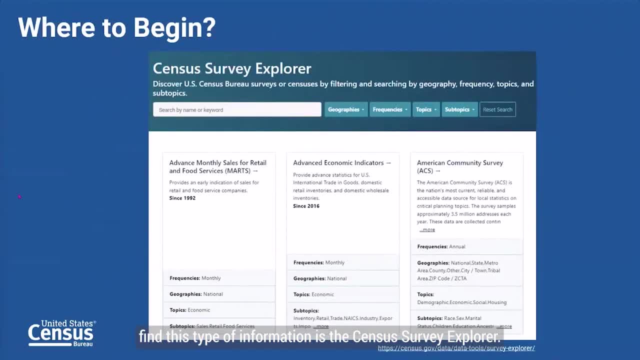 the Census Survey Explorer. This tool will provide you with a brief description of the survey, including the geography it covers, the frequency it occurs, topics as well as subtopics. You can also search by keyword. For example, if you type in education in the search bar, it will bring up the relevant 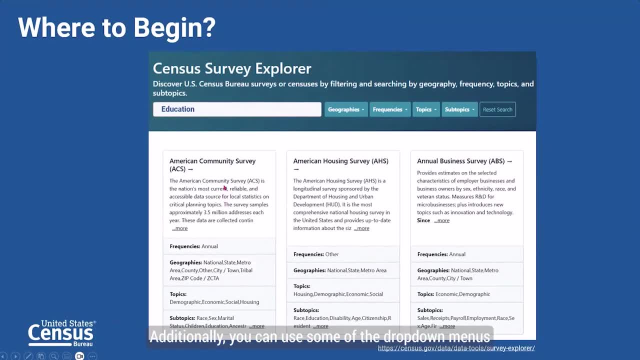 survey corresponding to your query. Thank you, Thank you. Thank you, Hilary. Thank you Jason. Thank you, Vanessa. Thank you. Okay, So the Census Survey ПK includes data that are available on censusgov. This is where you can find the data. that's part of the Census Survey, which is in the 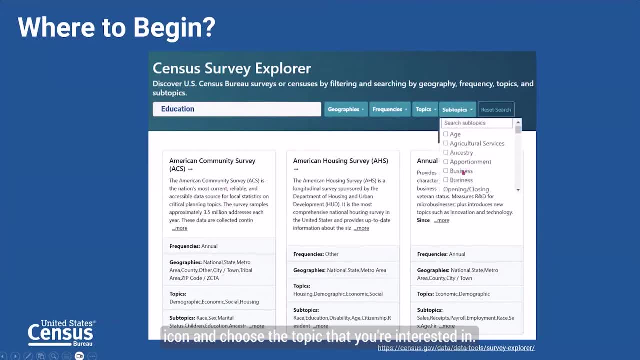 table that you can see on your screen, And you can also select the subject that you're interested in, And that should also bring up the result based on your query. You can also click on the drop-down icon and choose the topic that you're interested. 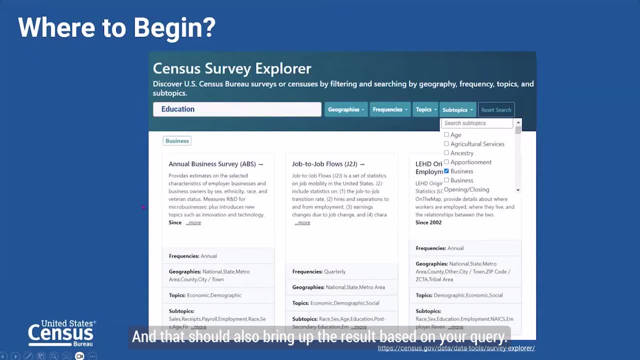 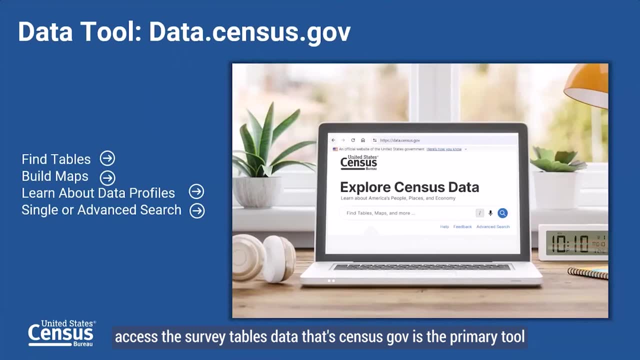 in and that should also bring up the result based on your query. Now to access the Survey Tables: datacensusgov is the primary tool that the Bureau has. Using datacensusgov, you can find tables, build maps, access data profiles. You also have the 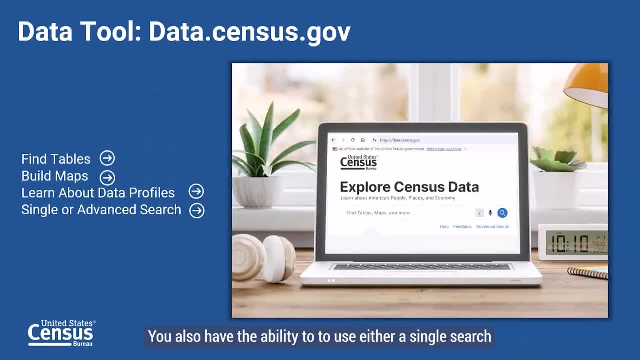 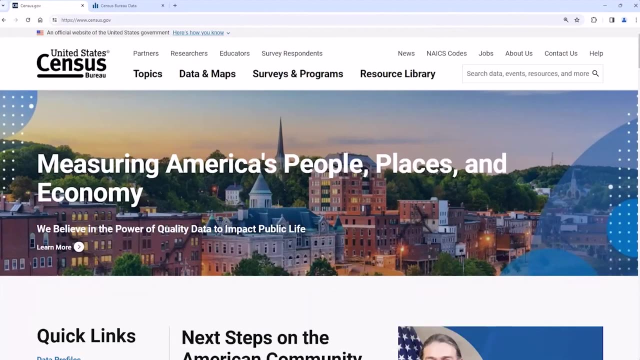 ability to use either the single search, by using keywords, or the advanced search for a more guided approach. So, in order for us to get into datacensusgov, you can navigate from our site, which is censusgov site, by going into the data and maps ribbon and then hovering over data tools. 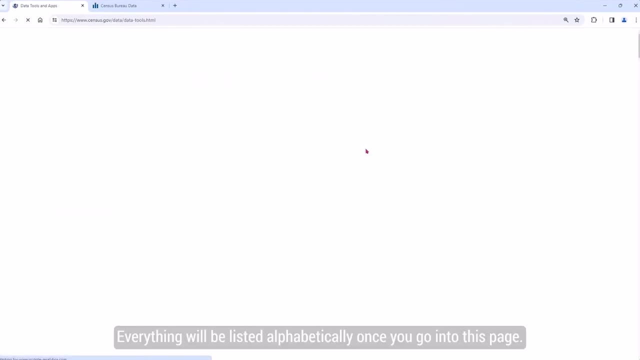 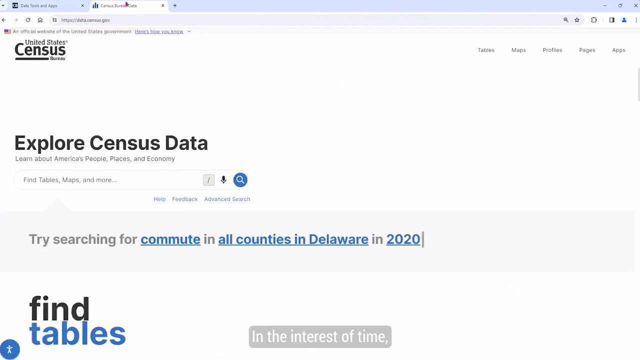 and apps. Everything will be listed alphabetically once you go into this page. However, I've already pre-loaded datacensusgov. in the interest of time, You can also type it into your web browser as datacensusgov. So from here we will begin by doing the advanced search option. 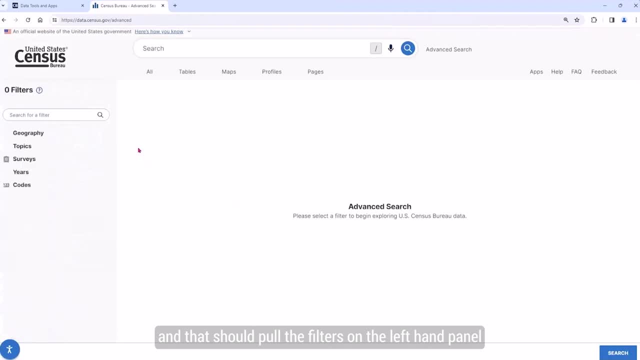 And that should pull the filters on the left-hand panel for you to choose from. So we will start with the geography filter And the team wanted to compare both the nation numbers as well as the state, So we will go ahead and choose the nation and click on the box on the US. 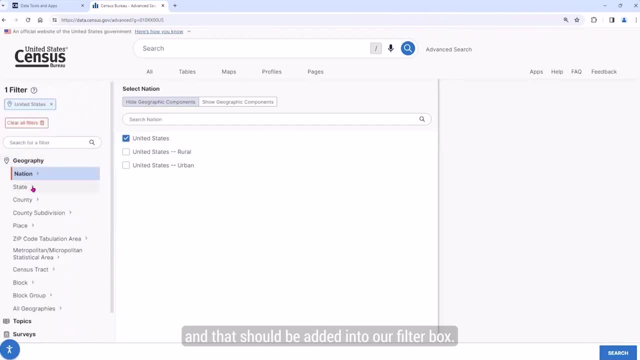 And that should be added into our filter box. And then we'll go ahead and also choose the state as part of our geography, And they were interested also in California, So we'll add and check that box as well. Now the next filter that we will use: 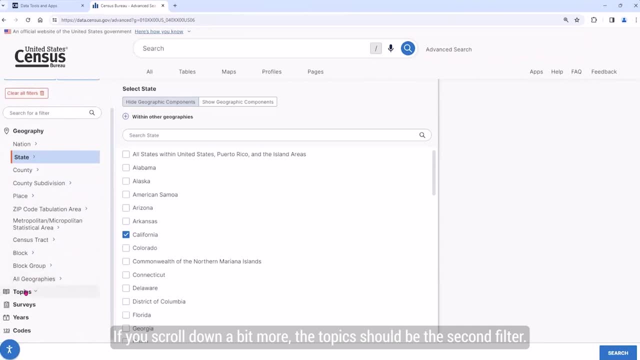 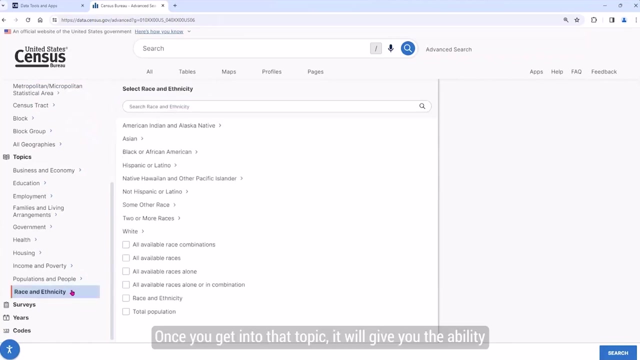 is the topics filter. If you scroll down a bit more, the topics should be the second filter. There is an icon to expand and collapse the filters, And so race would be here at the bottom of the list of topics. Once you get into that topic, it will give you the ability to 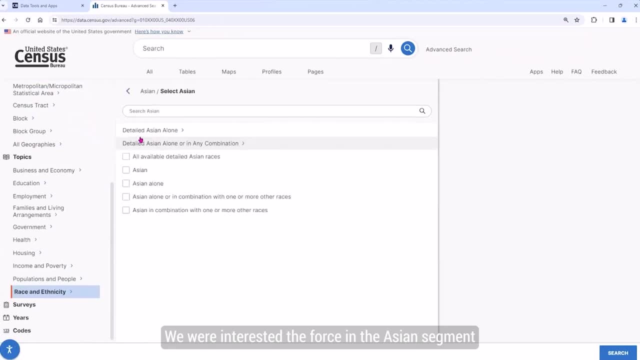 choose the different race. We were interested, of course, in the Asian segment And for this particular demonstration we will just do the Asian alone. So now that we've added those filters- as you can see, you have three on the left- we go ahead and. 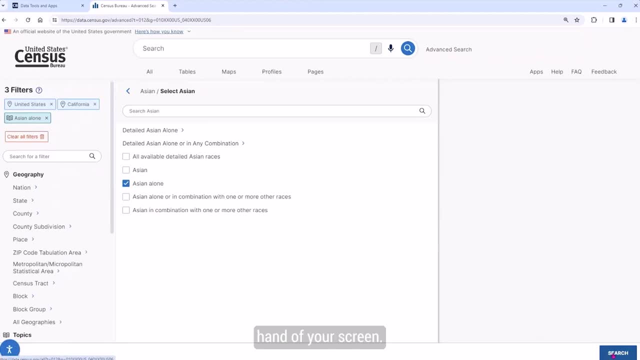 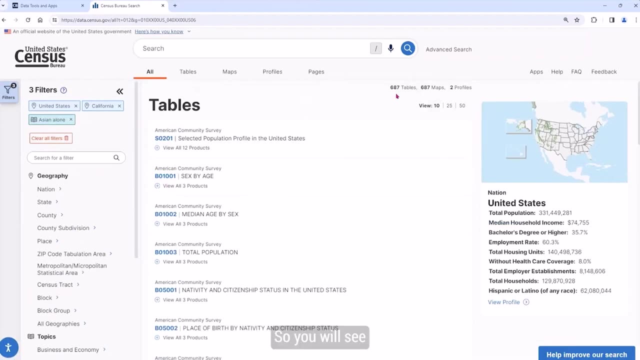 click the search button on the very bottom right-hand of your screen And that should generate for us the various tables related to our filters. So you will see it has generated 687 tables, corresponding to 687 maps and two profiles. We are interested in this very first table, the S0201, which is the 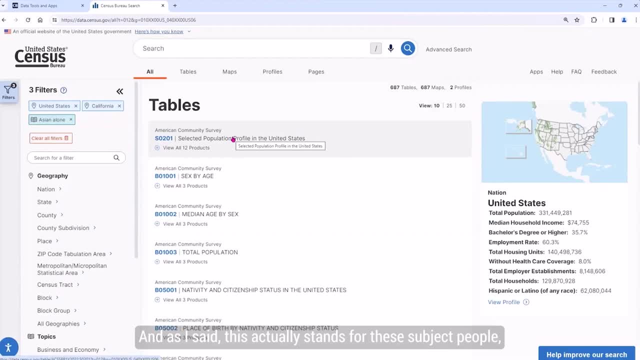 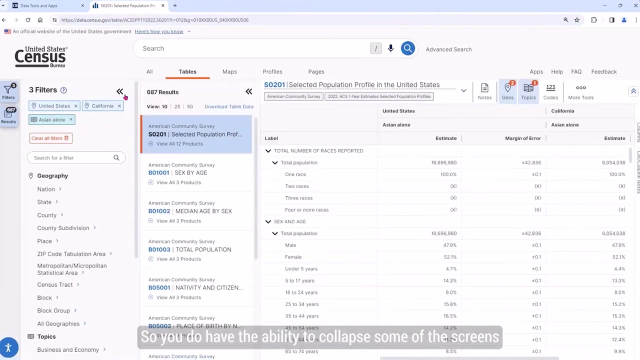 selected population profile. And, as Anne said, S actually stands for the subject tables, which means it presents a span of information on an ACS subject in both an estimate and percentage format. So you do have the ability to collapse some of the screens so that you can expand the. 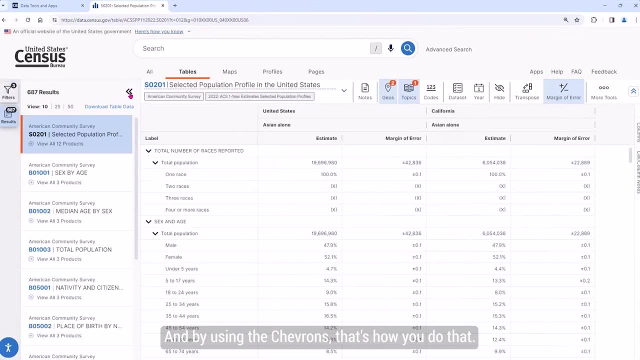 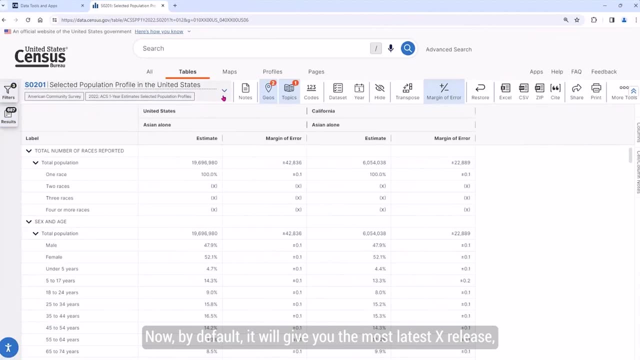 view of your data and by using the chevrons. that's how you do that. Now, by default, it will give you the most latest ACS release, which is right now the 2022.. One-year estimates is what we have here, but you do have the option of using the drop-down menu and you can go back to the. 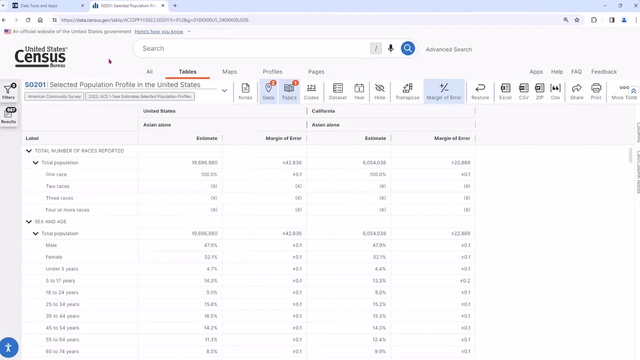 different vintages, all the way to 2010.. Now, this table does give you your chosen geography and you can see that it's a little bit different. So you can see that it's a little different in geography, which is the nation as well as the state, and then we have the variables. 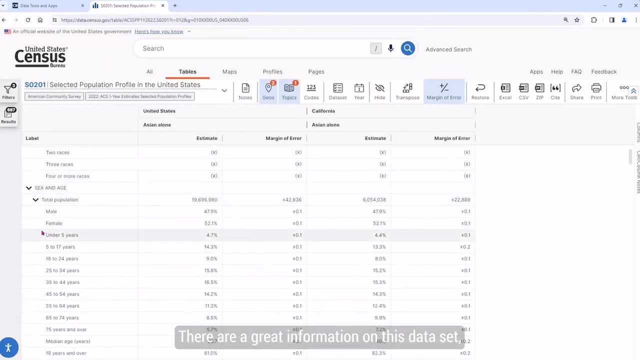 on the left-hand corner. There are a great information on this data set, but I just wanted to highlight a couple of them. For instance, here, when we come to the age groups, you will see those who are 18 years and older makes up the largest group of the Asian population, with almost 16. 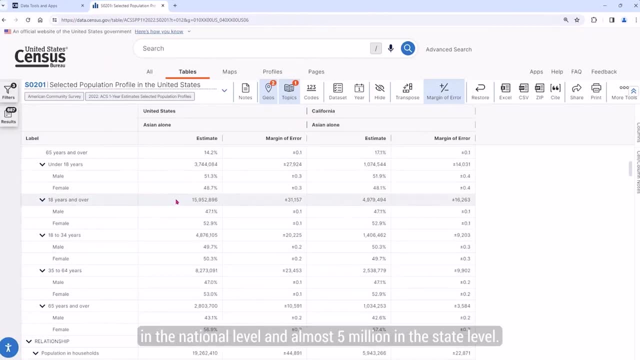 million in the national level and almost 5 million in the state level. I'm going to take out the margin of error right now. So I'm going to take out the margin of error right now and I'm going to so that we can just compare our geography a bit better And if you scroll down a bit more into, 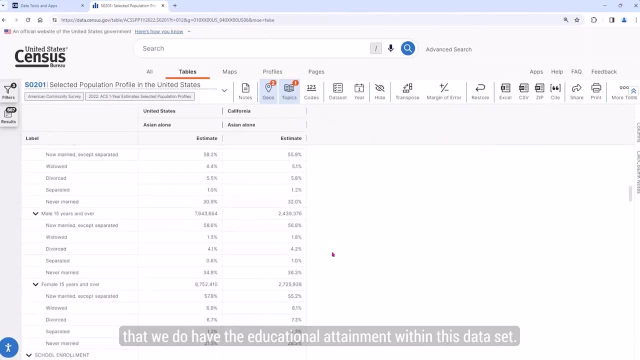 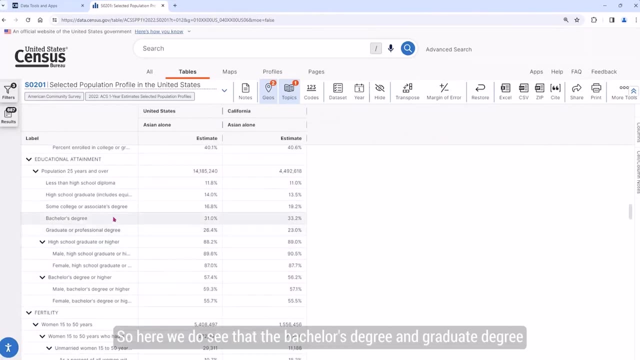 this dataset, you will find that we do have the educational attainment within this dataset. So here we do see that the bachelor's degree and graduate degree actually make up the top two when it comes to educational attainment for the Asian population. If we drill down a bit more, 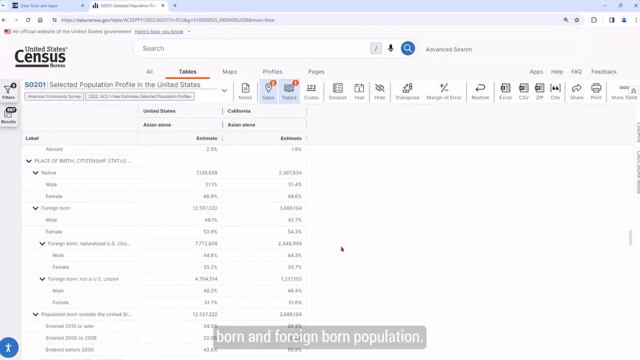 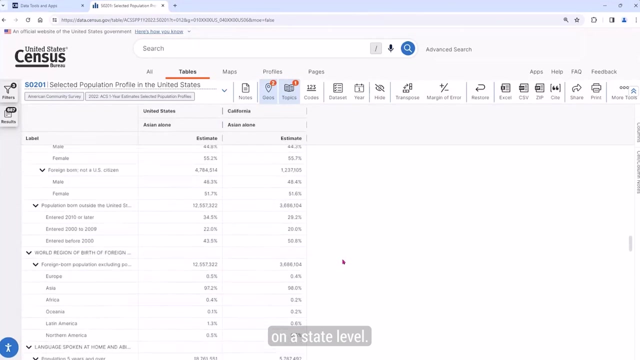 we will have a bit more information in terms of the native-born and foreign-born population. A great number of Asians are actually foreign-born, with more than 12 million on the national level and more than 3 million on the state level. This dataset will also provide you with information in terms of the occupation. 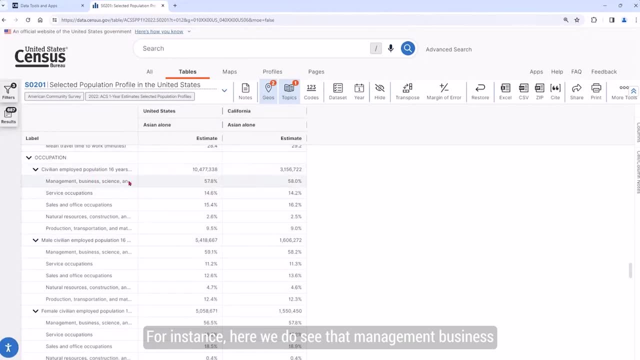 for the Asian segment, For instance. here we do see that management, business and science and arts occupation are actually the top two in terms of where the Asian community is engaged in. If you're not able to see the description of the variable, all you need. 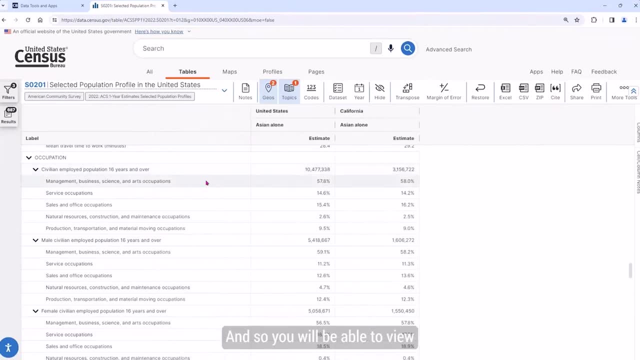 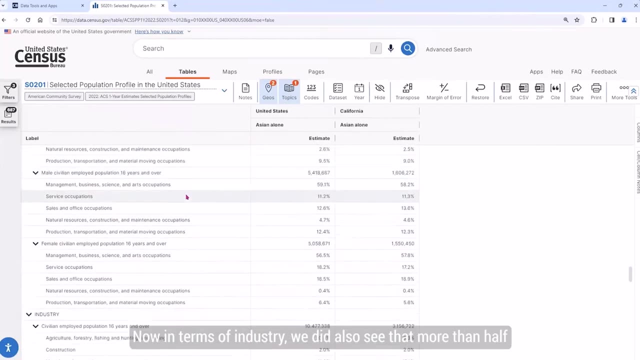 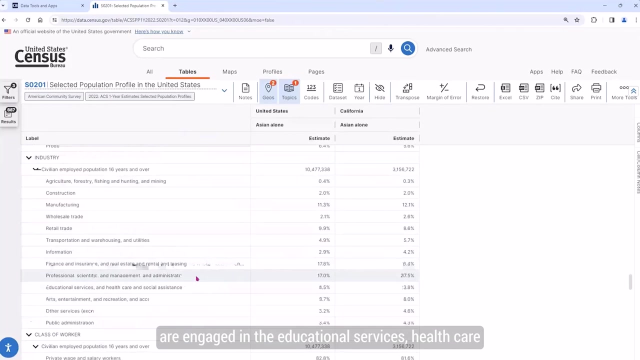 to do is to expand the column, and so you will be able to view the explanation in terms of what that variable is Now. in terms of industry, we did also see that more than half of the Asian are engaged in the educational services, health care and social assistance. These 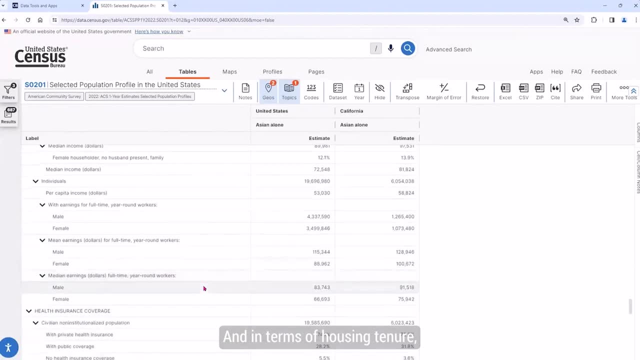 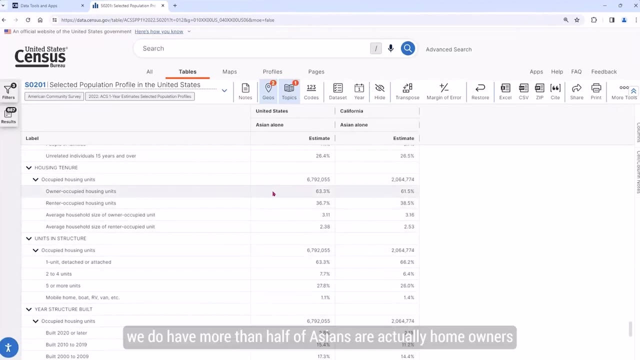 are the top industries where the Asian community are employed in, And then in terms of housing tenure, we do also have that information within this dataset. As you can see, here we do have more than half of Asians are actually homeowners versus renters, And this is reflected in both the 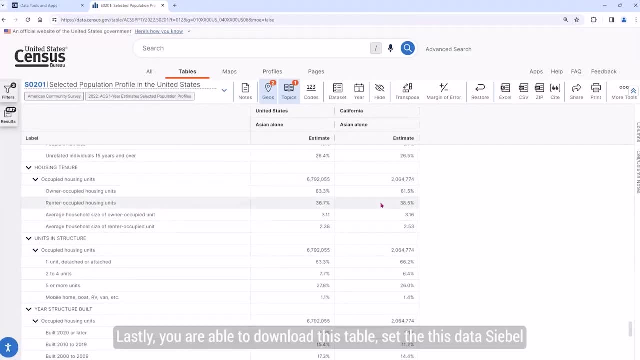 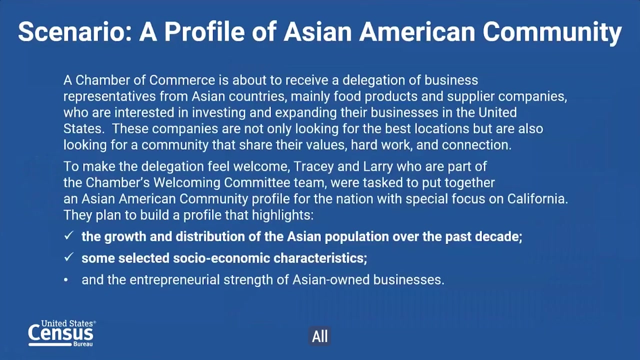 well as the state level. lastly, you are able to download this table. set this data table by using our icons on ribbon. you can download through an excel, csb, zip file, or share, or even print, depending on your preference. all right, with that table, the s0201, we found we have fulfilled the second item on our scenarios. 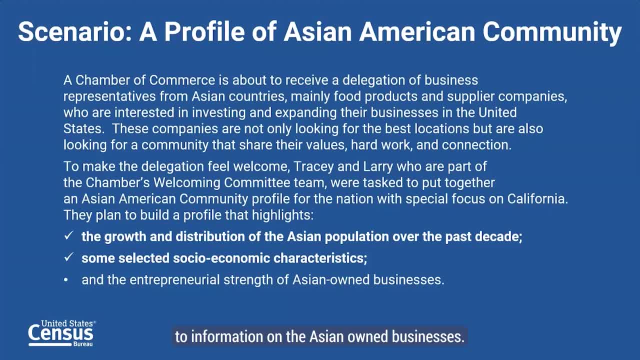 list. our next task is to look for the information on the asian-owned businesses, and there are several census surveys that can provide you with this data. for instance, one is the annual business survey, or the abs. it's really a great source of information for the asian-owned businesses. 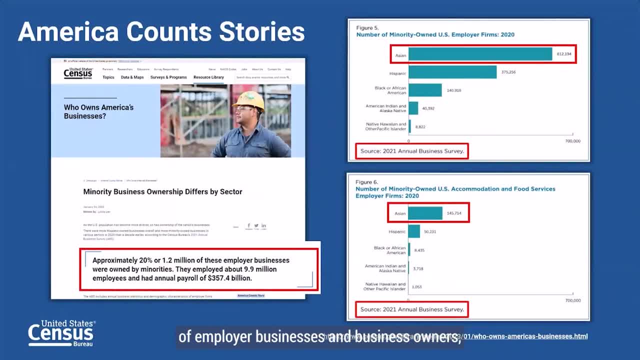 and that survey will allow you to choose and share your own work ar subjects. please just do so on those websites that you help. your survey be held in chapter 6. so all of this data of our surveillance activity failed to help lead and organize the activity. another question that we have for students: 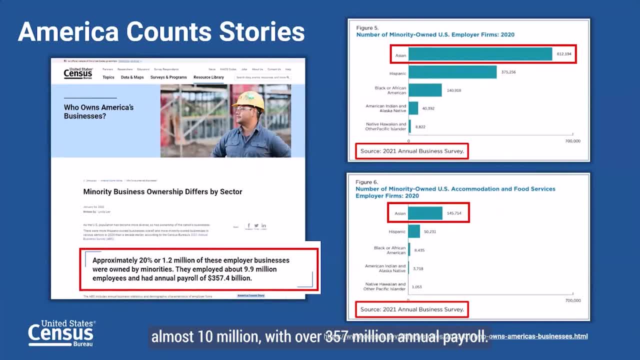 is whether the other graphic, here provisions are required to work, do different Maine Floridamaine, Florida or Maine Florida, within the sort of recording criteria that we, Syndex, may give in order to structure our survey. businesses employ almost 10 million with over 357 billion in annual payroll. In fact, there are more. 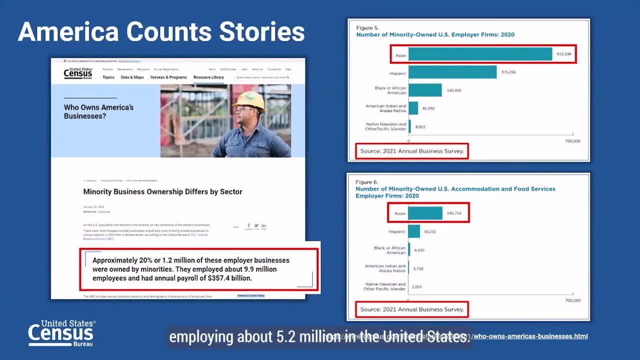 than 600,000 Asian-owned businesses, employing about 5.2 million in the United States. This is the highest among all minority groups. A large share of the Asian-owned firms, approximately 23.8 percent, were in the accommodation and food services sector. The number of Asian-owned 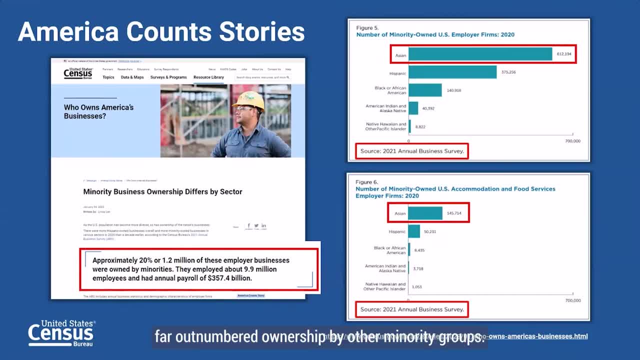 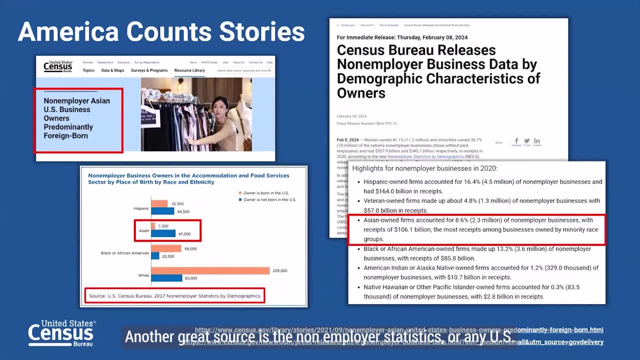 businesses in this sector far outnumbered ownership by other minority groups. Another great source is the Non-Employer Statistics, or NES for short, which provides information on non-employer businesses. These are businesses that have no paid employees and have an annual business receipt of a thousand dollars or more, and you can think of them generally as 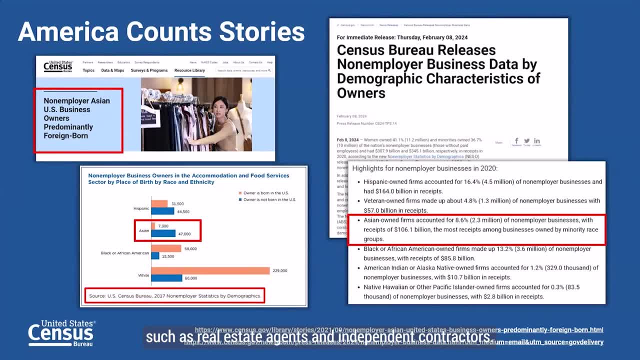 small businesses, such as real estate, real estate companies or real estate companies, agents and independent contractors. Another great article from our America Counts stories shares with us that in 2017, NES release: Asian non-employer business owners are predominantly foreign-born. For example, this is reflected on the accommodation and food service industry. which has significantly higher foreign-born versus native-born Asian non-employer business owners. Additionally, in the latest NES release, the report shares that in 2020, Asian-owned firms accounted for 8.6% of all non-employer businesses- Again the highest. 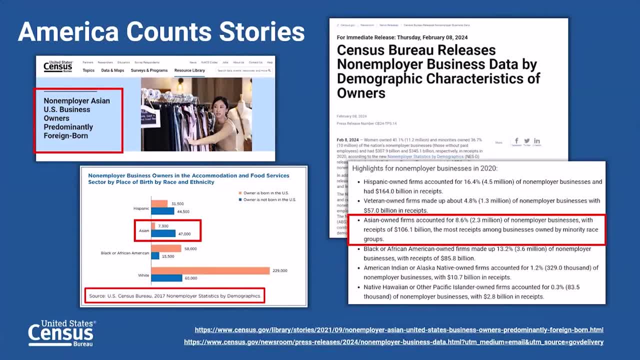 among business-owned by minority groups. As you can tell, this information correlates to what we saw earlier with our table S0201.. It did show us that the breakdown of the Asian population was significantly higher than the number of non-employer businesses, As being majority foreign-born versus native-born. 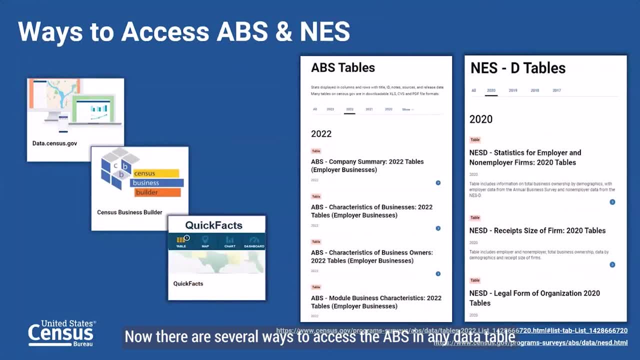 Now there are several ways to access the ABS and NES data table sets, and here are just a couple of the tools on the left hand. Additionally, we do have ABS and NES D table list, which quickly leads you to the data sets. For instance, to find the basic tables, you can go. 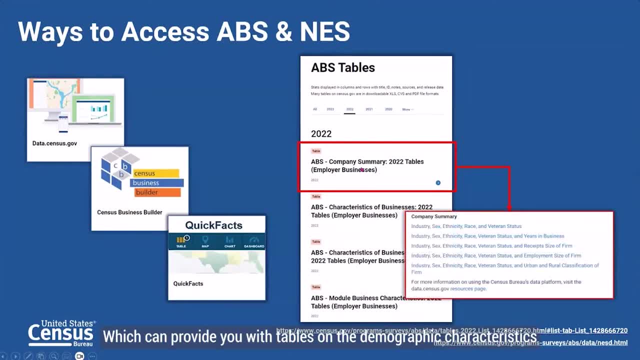 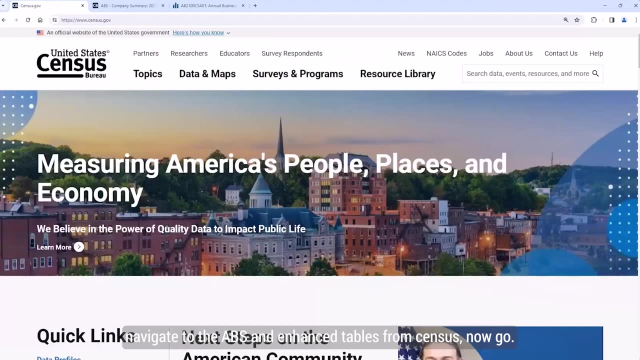 to the company summary tables. This table is probably a little bit different from the one that we had before. This is the table which can provide you with tables on the demographic characteristics of business owners by race, sex, ethnicity and veteran status. To navigate to the ABS and NES tables from censusgov, all you need to do is go to the. 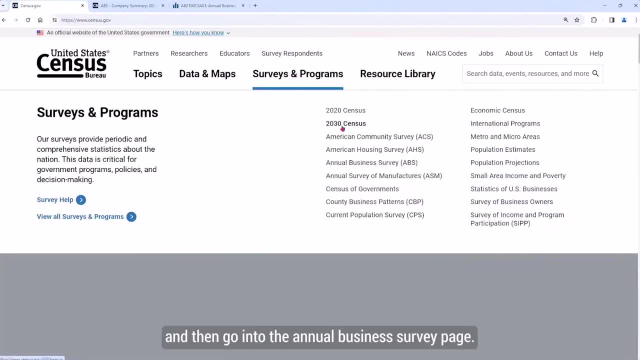 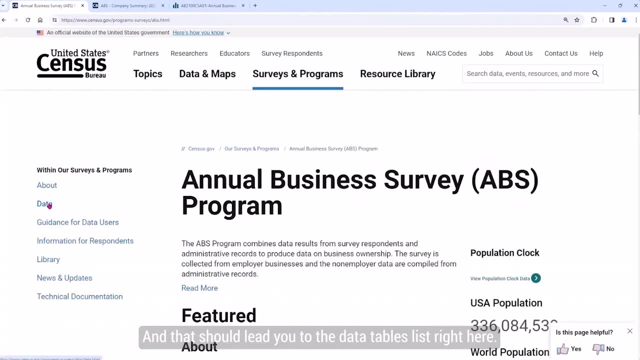 surveys and programs ribbon and then go into the annual business survey page. That should lead you to the data table and table data set. This is available here. You can access the job analysis tables list right here, But I've already pre-opened it, so in the interest of time, here is the list. 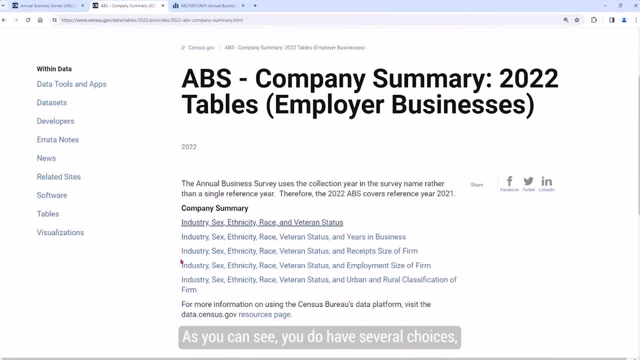 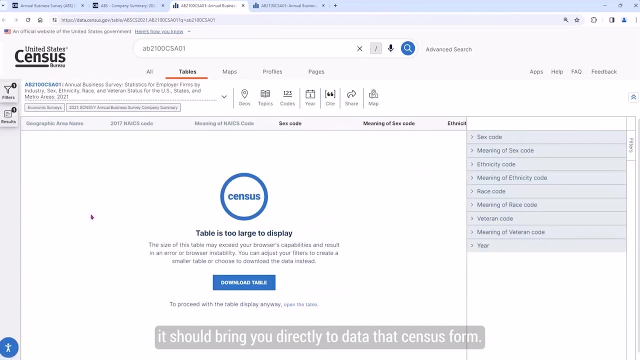 under the company summary. As you can see, you do have several choices, but what we want to do is go into the very first one, which is the basic data table set, and once you click into that, it should bring you directly to datacensusgov. So, here from the landing page, it does provide you with. 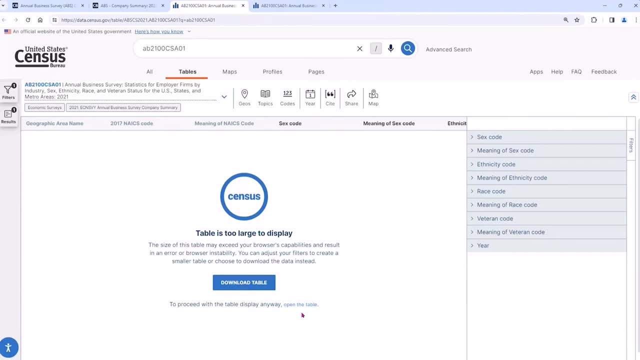 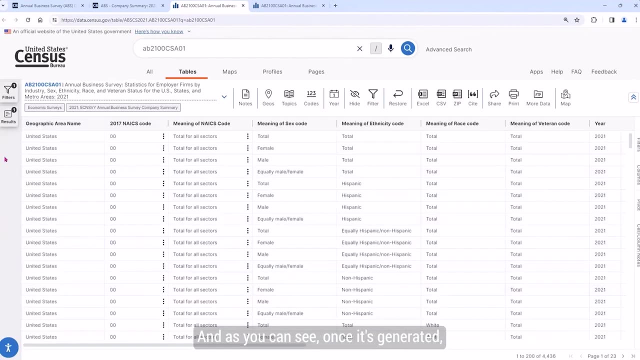 two options: either to download the table or open the table. We will go ahead and open the table and, as you can see, once it's generated, it will provide you with the area by default as entire nation. You have the NAICS code, the two-digit NAICS code, together with the meaning. 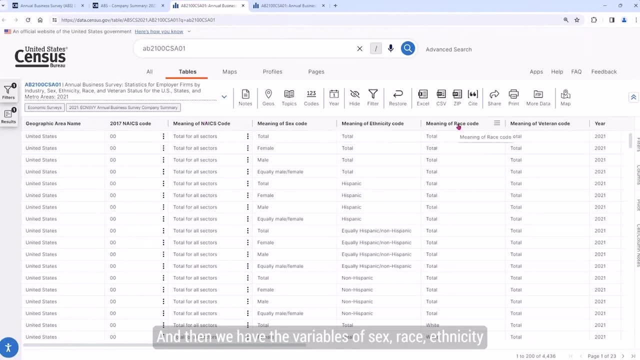 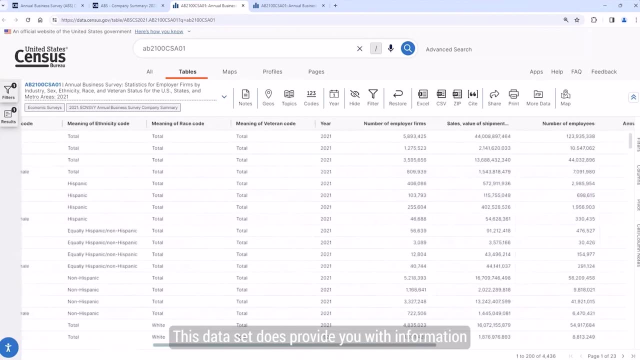 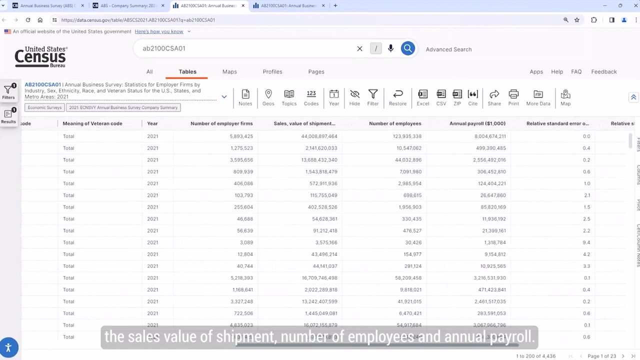 and then we have the variables of the sex, race, ethnicity and veteran code. If you scroll to the right, the scroll bar is at the bottom of your screen. This data set does provide you with information on the number of employer firms, the sales value of shipment, number of employees. 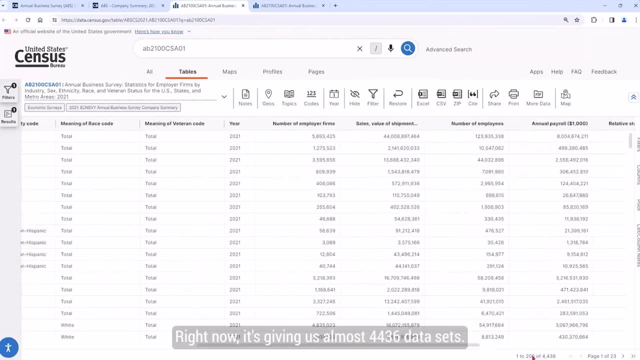 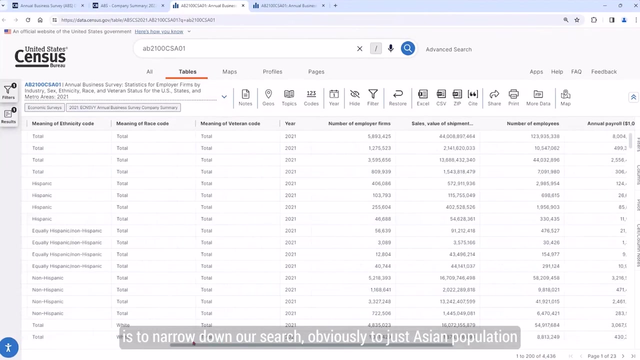 and annual payroll. Right now, it's giving us almost 4,436 data sets. if you look here at the bottom right hand of the screen, This is based on the 2021 ABS release, So what we want to do is to narrow down our search. 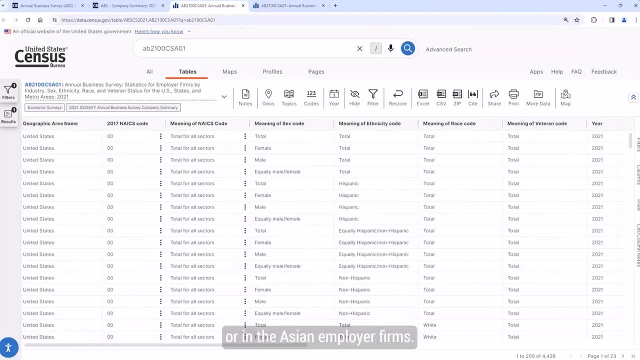 obviously to just the Asian population or the Asian employer firms. and what we will do is to filter these four columns here by just clicking on the icon for the filter and going into the funnel filter and we will deselect and just select the totals for the sex and apply. 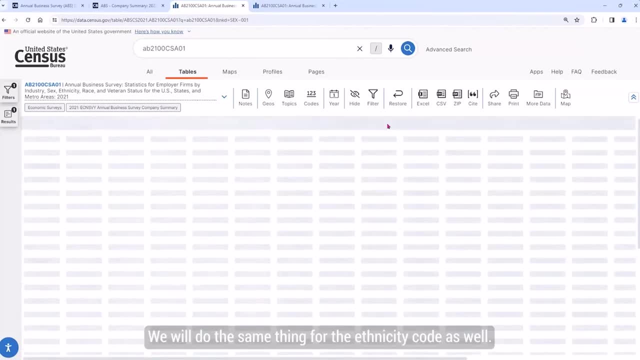 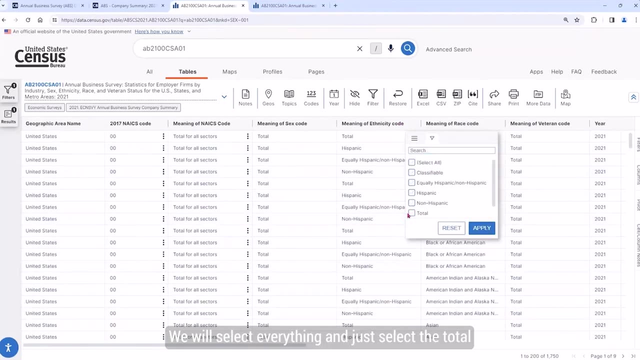 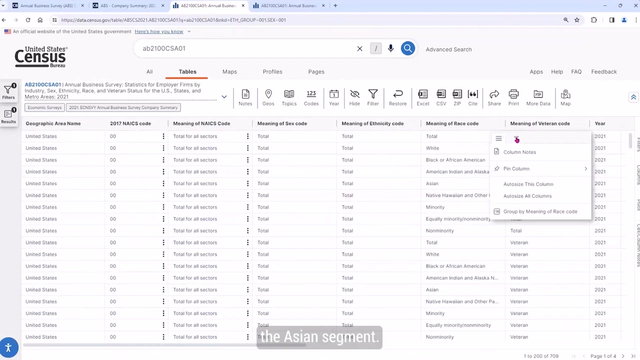 We will do the same thing for the ethnicity code as well. We will go ahead and go into our filter icon. we will deselect everything and just select the total, And then for the race. we want to make sure that this will only showcase the Asian segment, So we will go. 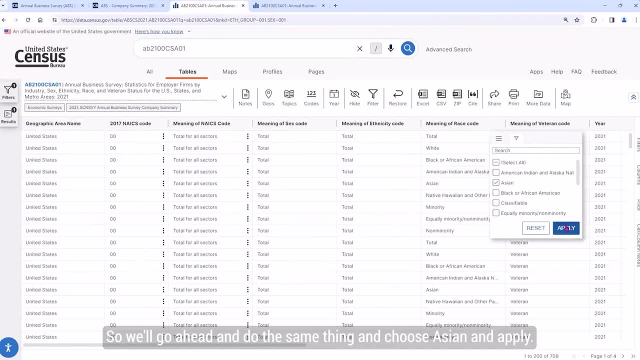 ahead and do the same thing and choose Asian and apply. And then, lastly, we'll just go ahead and just make totals for the same thing, for the veteran price. So we will go ahead and do this, I'll just make taughtles, which means that the бу ethanol will only do so for each of these three드� gonlidel. than we'll go ahead and do the same thing and choose Asian and apply, And then, lastly, we'll just go ahead and just make totals or the same thing for that veteran craft. So you won't want to do that. We want to make totals just to indicate the advantages of having specific墨. 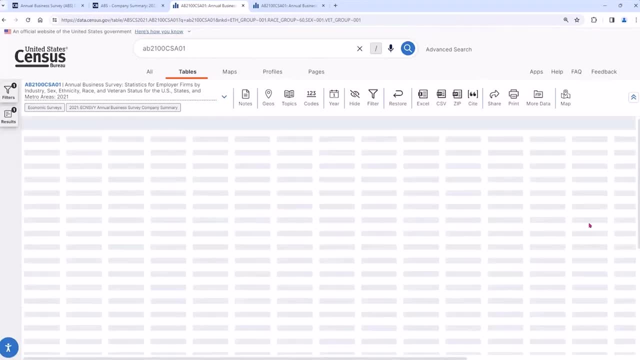 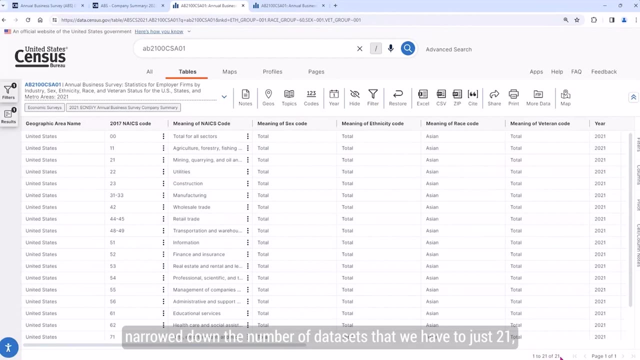 for the veteran code as well. So once we've done that, you will see that we have now narrowed down the number of data sets that we have to just 21,, which shows us the information on the total sectors as well as the different. 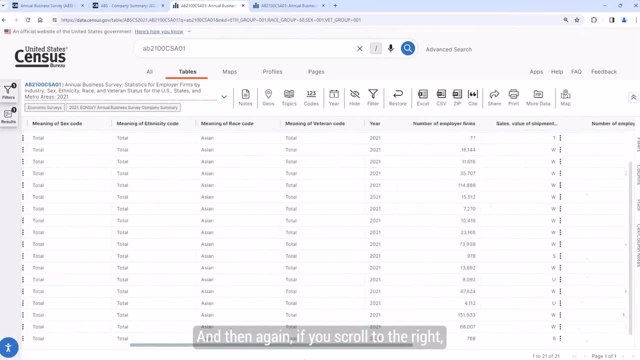 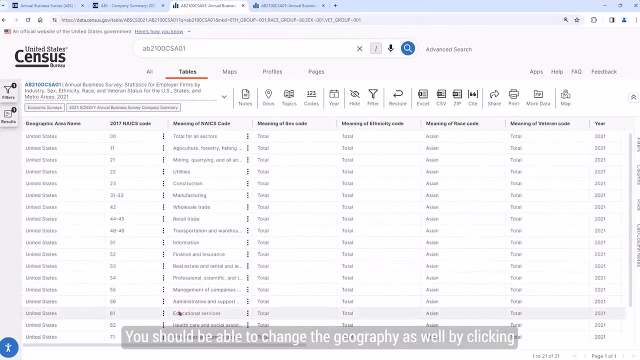 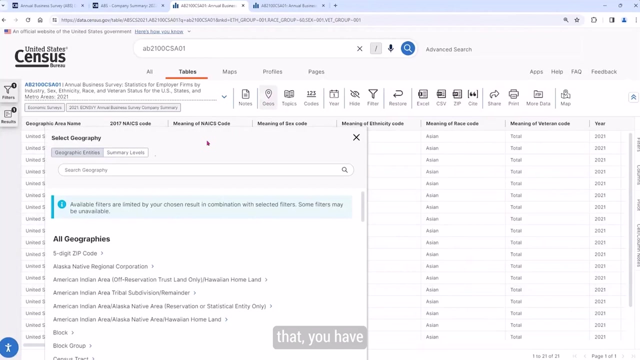 NAICS code of interest And then again, if you scroll to the right, you will see the different data sets available for you. You should be able to change the geography as well by clicking on the geography icon. Once you do that, you have the option of choosing. 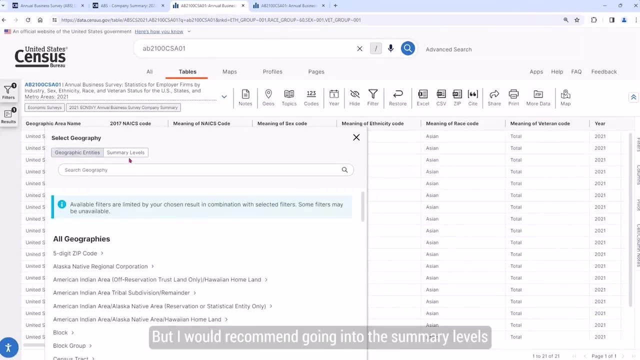 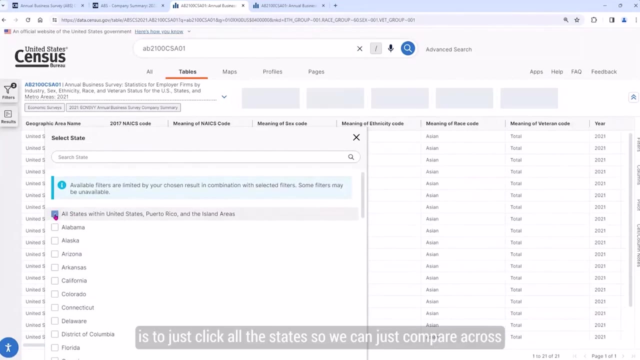 the different geographic entities of the census, but I would recommend going into the summary levels, as this already limits your choice based on this particular data set. We'll go ahead and choose the state level, And what we want to do is to just select all the states. 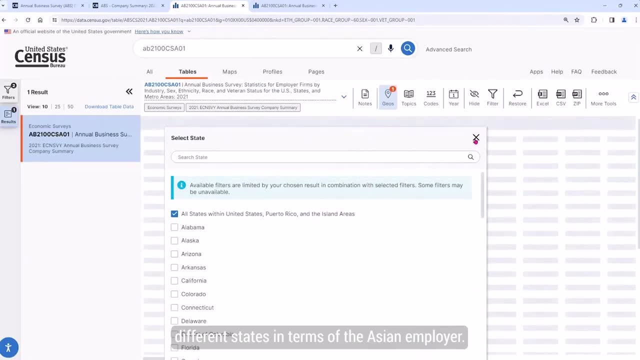 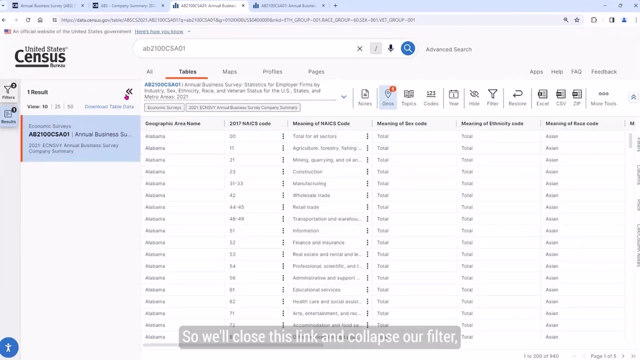 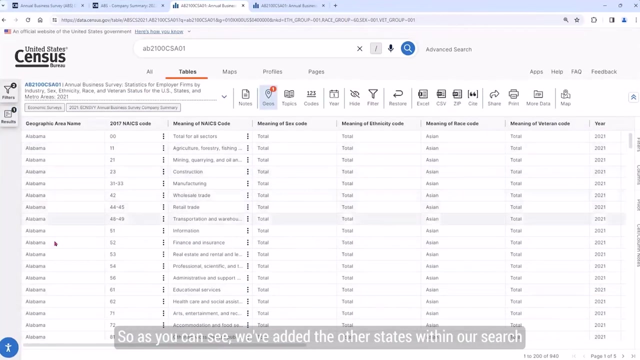 so we can just compare across the different states in terms of the Asian employer firms. So we'll close this link and collapse our filter. Make sure that we view our table better this way around. So, as you can see, we've added the other states. 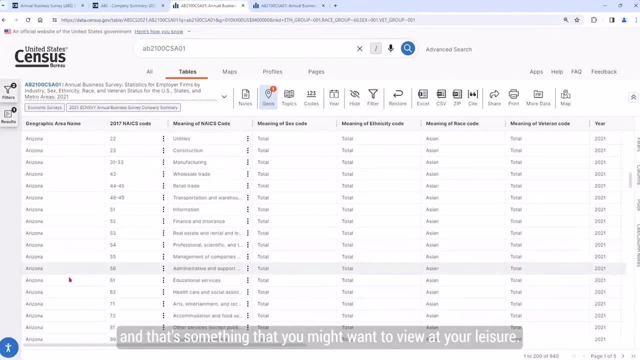 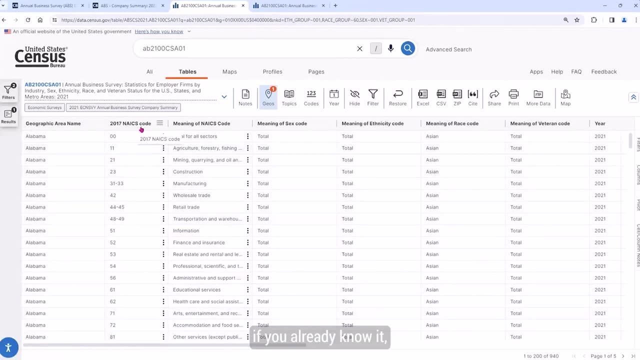 within our search, and that's something that you might want to view at your leisure. Now you also have the option of filtering by NAICS code, if you already know it, or you can do it by the meaning of the NAICS code. 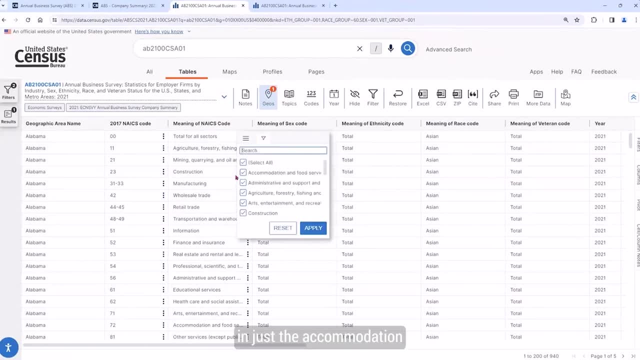 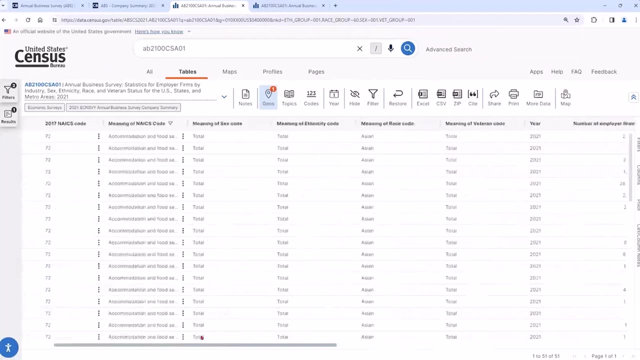 So, for instance, if the chamber was interested in just the accommodation and food services, all they need to do is just select that filter and apply it, And that should give you just that particular industry in terms of information. One great thing about this table. 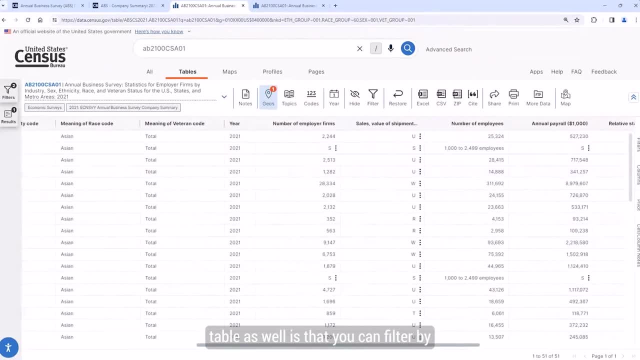 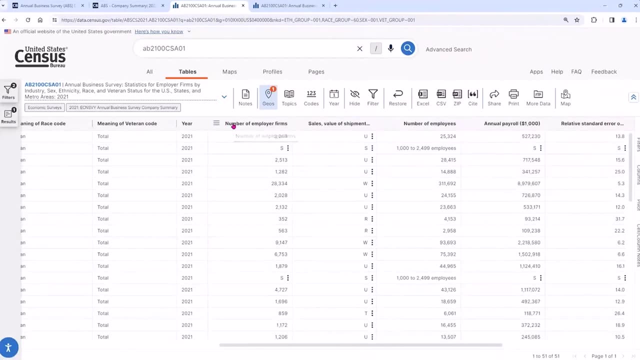 as well is that you can filter by the ascending or descending order. So if you wanted to do that, you can just click on the text and you will see that there is an arrow generated. So, basically, you filtered it by ascending order or, if you wanted, descending order. 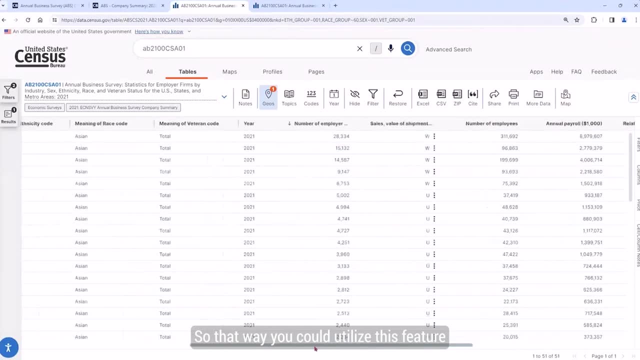 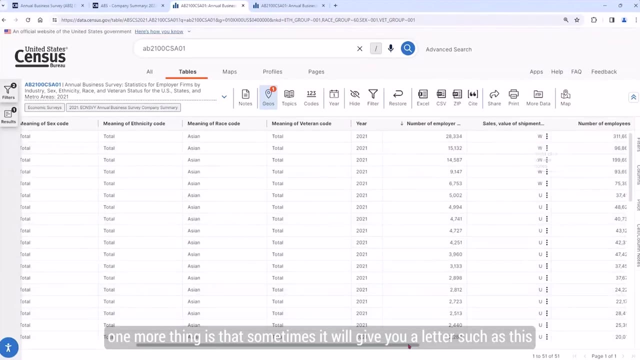 So that way you could utilize this feature if you wanted to. One more thing is that sometimes it will give you a letter such as this and doesn't give you a number. What you need to do is just right click on or click on the cell. 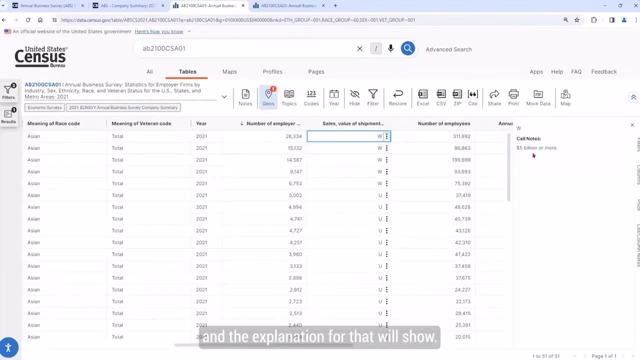 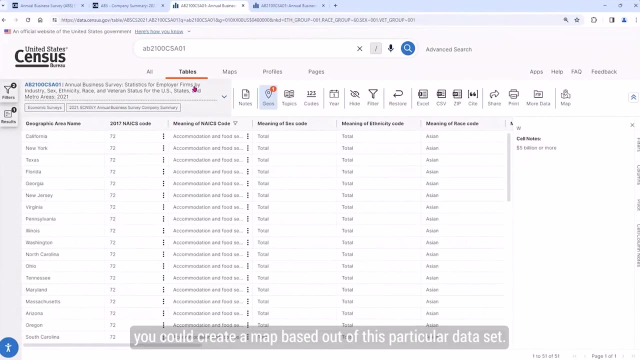 and do a right click and the cell mode should appear and the explanation for that will show. Lastly, I wanted to share how you could create a map based out of this particular data set. All you need to do is just go into the maps feature within the ribbon. 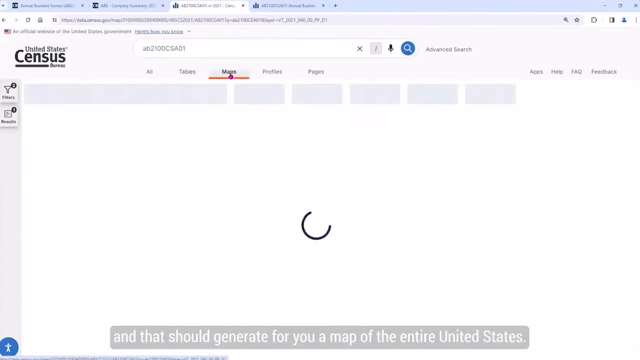 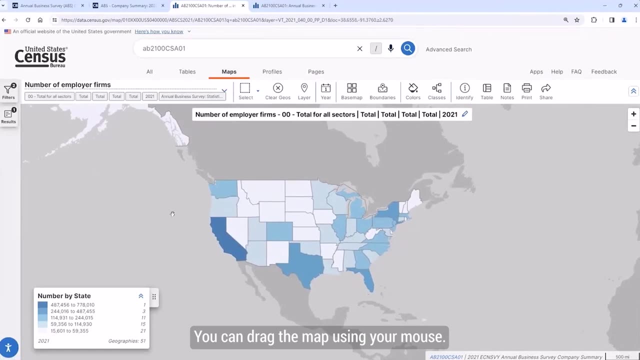 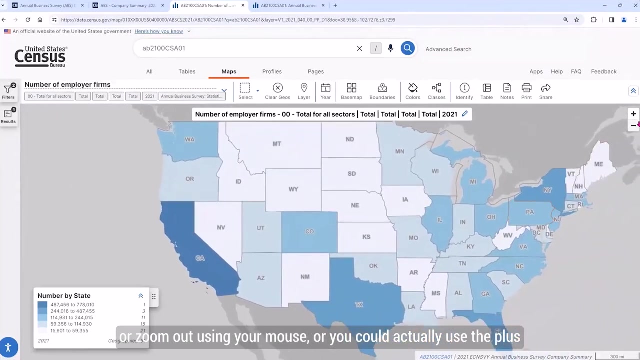 on the top and click on the maps And that should generate for you a map of the entire map. So if you're in the United States, you can drag the map using your mouse, You can zoom in or zoom out using your mouse or you could actually use the plus. 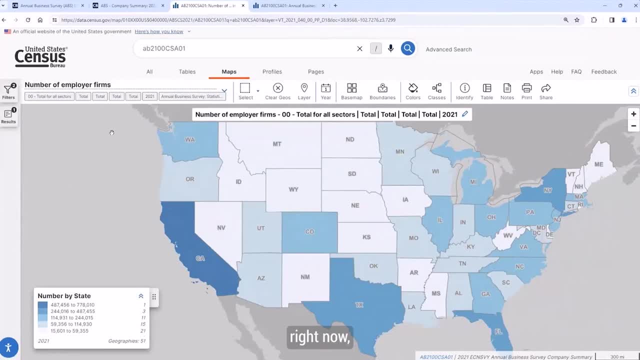 or minus icon right here on the right hand panel of the screen. Right now, by default, it's just showing us the number of employer firms. There is a drop down menu to make sure that your selections are still applied. You have the option of changing that if you wanted. 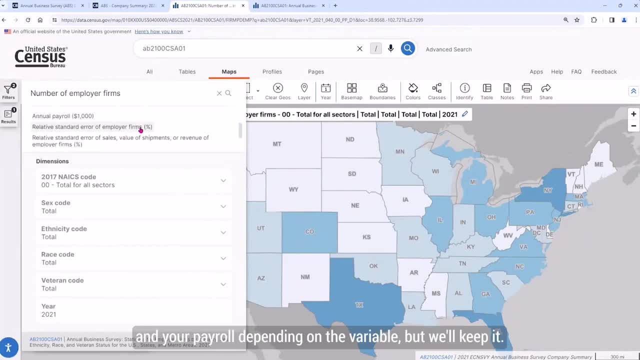 to show the sales value. number of employees, annual payroll, depending on the variable, but we'll keep it up. number of employer firms: We'll make sure that our next code right now is showing just the total sector, but if you wanted to, you can go back. 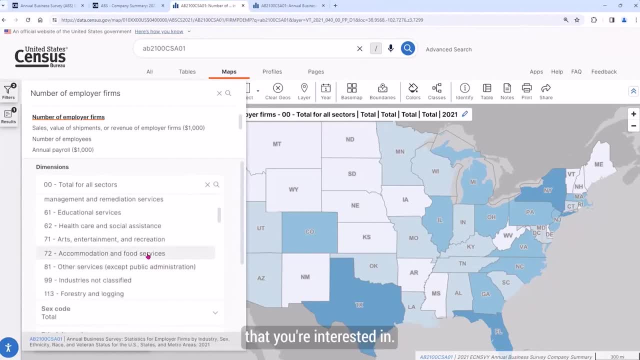 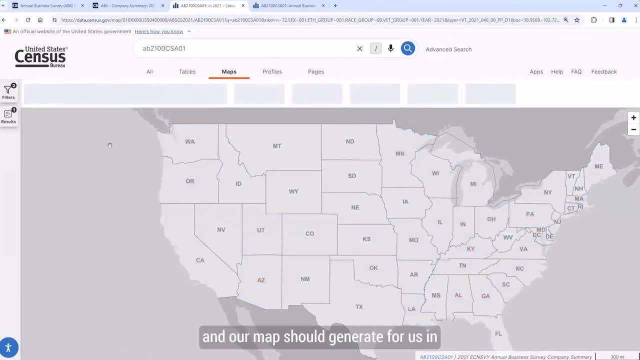 and filter it by the industry that you're interested in. For instance, we were looking at the accommodation and food services. We'll click on that And our map should generate for us in, based out of the filters that we've chosen. Let me try to reload that to be sure that it does try. 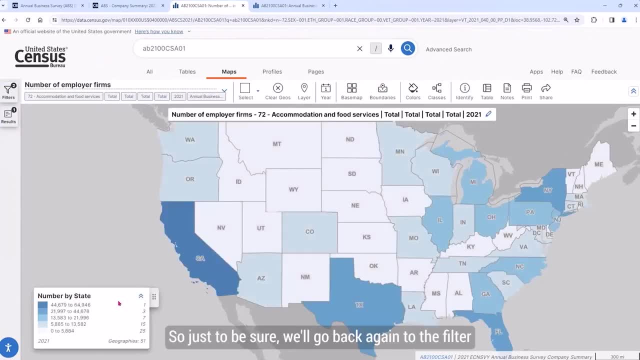 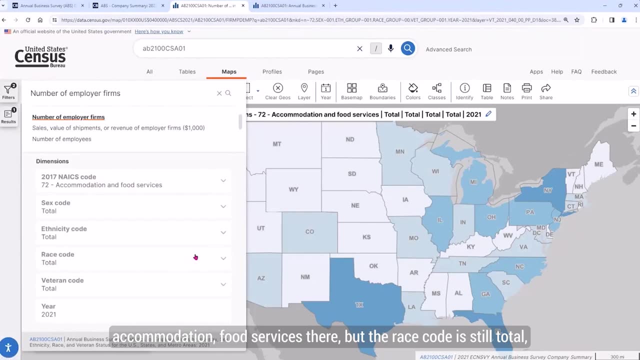 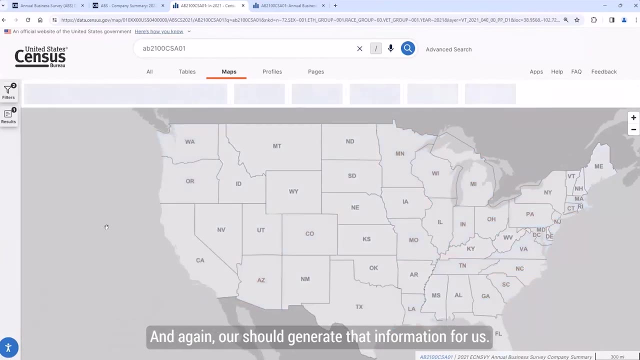 to give us that map again. So, just to be sure, we'll go back again to the filter accommodation and food services there. but the race code is still total, So we want to make sure that that is on the Asian segment And so we'll go ahead and choose Asian. 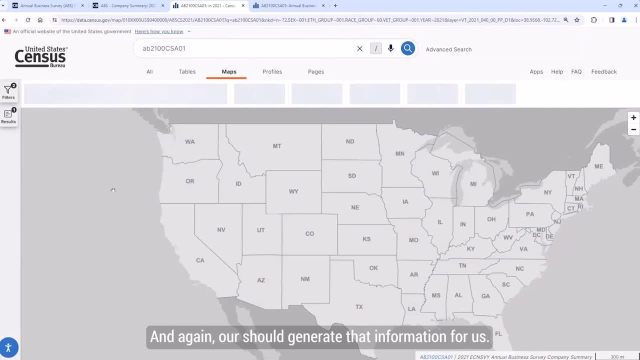 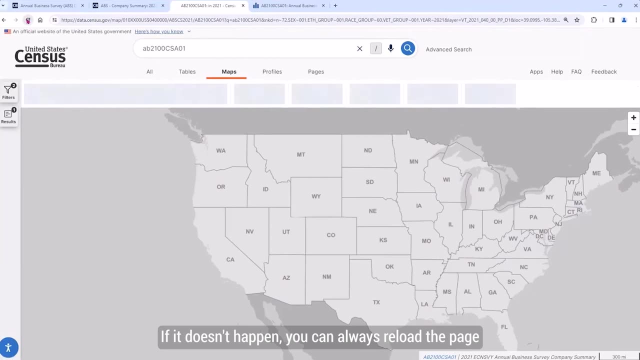 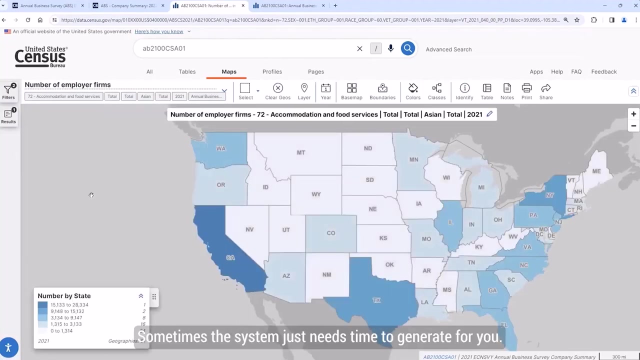 And again, our map should generate that information for us. If it doesn't happen, you can always do the reload the page to ensure that it does. sometimes the system just needs time to generate for you. So, as you can see, it has updated. 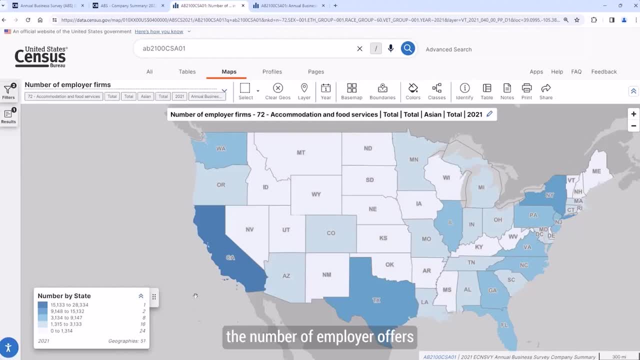 and it does show us that the number of employer firms, accommodation, food services for the Asian employer firms. the legend right here tells us that the darker shaded areas has the most number of Asian employer firms, with California being the top in terms of the number. 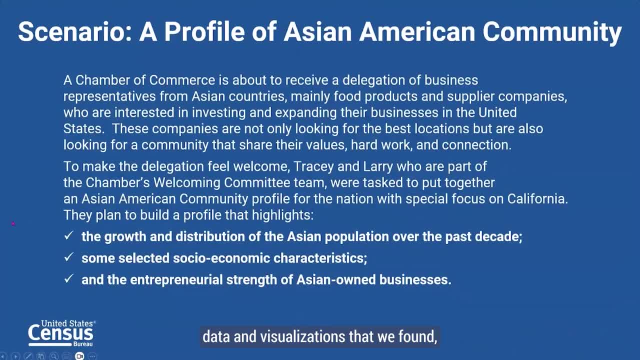 All right. given the data and visualizations that we found, all the information needed by the chamber team can now be put together for their Asian community profile. So we hope that with this scenario and demonstrations were helpful for you as you create your own report presentation. 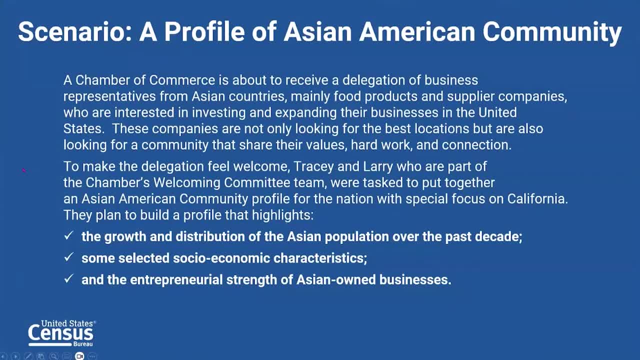 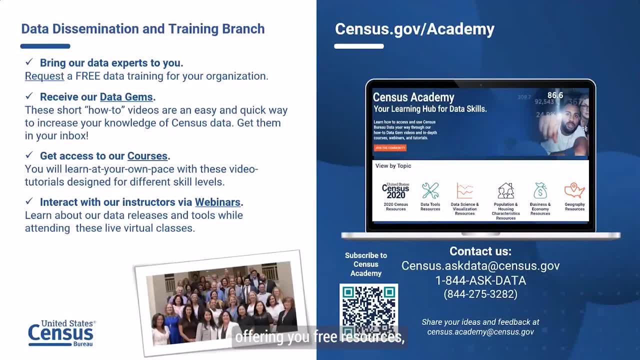 or community profile. So, just to close out, you can continue to learn more through our site, through the Census Academy, offering you free resources, including the data, gems and courses and various topics, all of which will allow you to learn at your own pace. 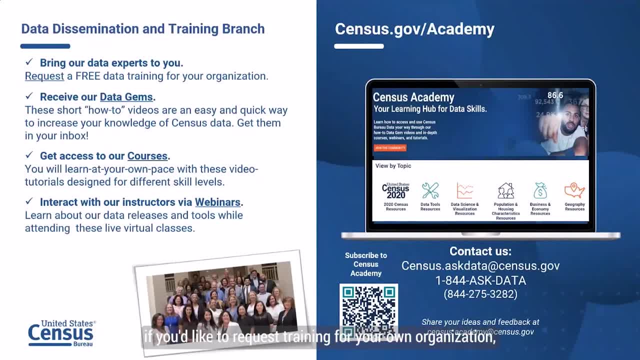 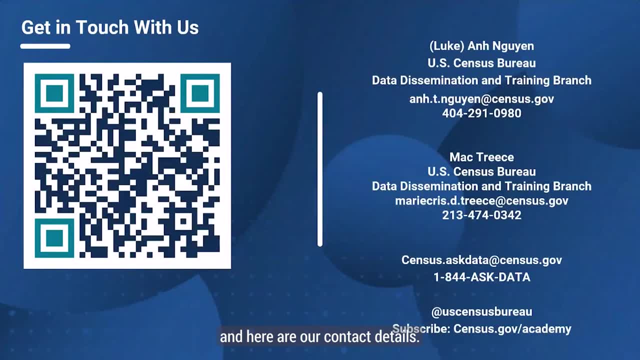 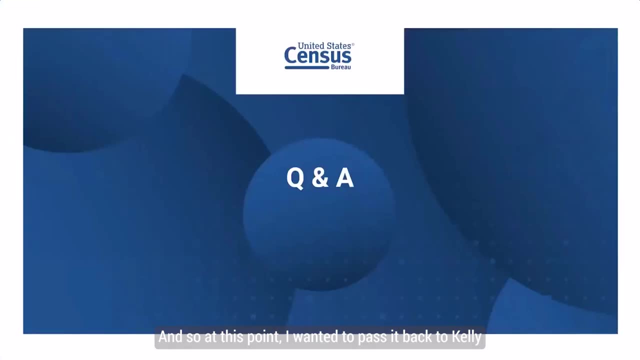 We also offer free data training. do reach out to us if you'd like to request training for your own organization, And here are our contact details. And so at this point I wanted to pass it back to Kelly and see if we do have any questions. 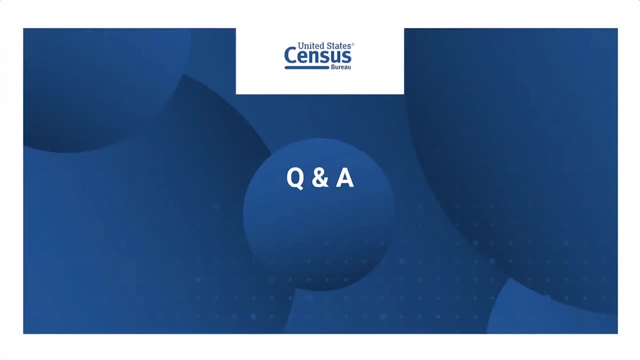 coming from our participants: Kelly. Hi, yes, Mac, I think we have time for a couple of very quick questions. The first question is: is county level data available for the Asian population? Yes, it is available. Thank you so much for that question. 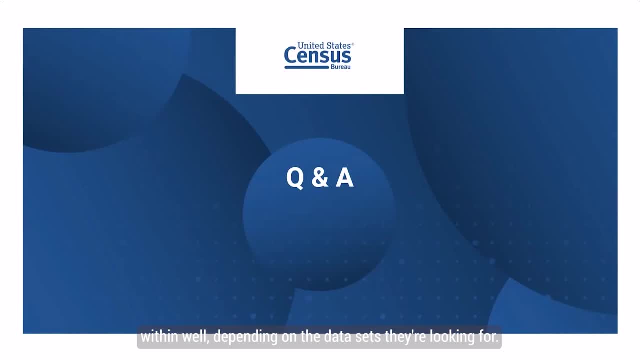 That would be within well, depending on the data sets they're looking for, but for the ones that we showed, it does have that information at the county level. With the acceptance, the adoption of the ABS as well as the NAS, there might be a different data set. 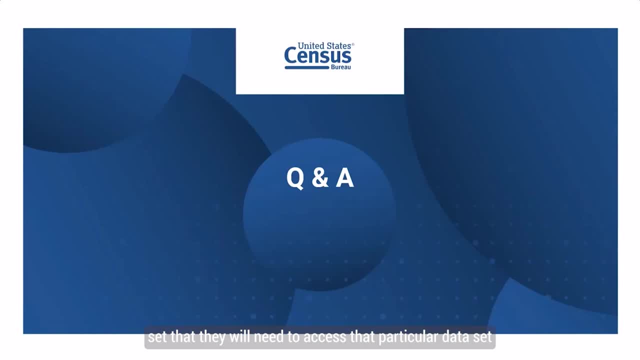 that they will need to access That particular data set. that I showed only goes to the state, nation and metro level. So if they can send us the question on the chat, we can definitely coordinate with them and show them how to navigate to the county level if needed. 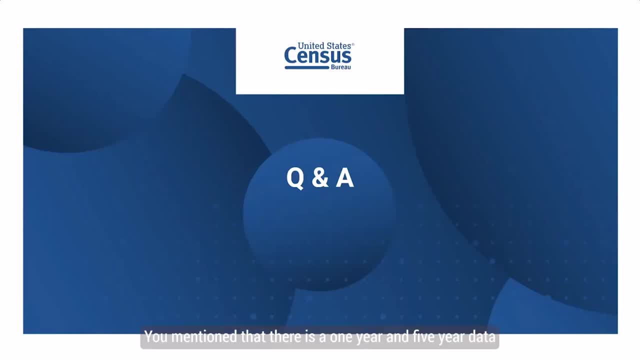 Okay, next question: You mentioned that there's a one-year and five-year data set from the American Community Survey. How often is the data from the American Community Survey released? Ron, did you want to take that one? The data set are being released yearly. 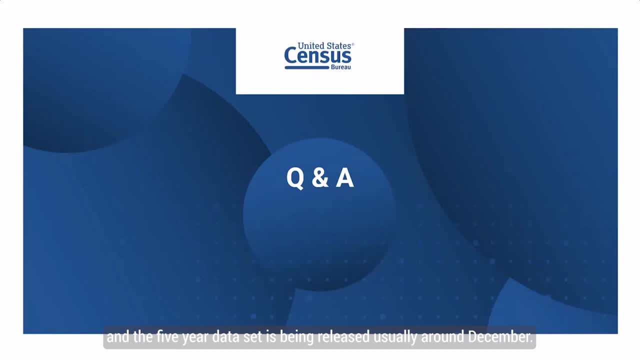 And the five-year data set is being released, usually around December. I don't have the. I would not say I don't have the data set. I don't have the data set. I'm not saying the exact date, but usually around December 19th, December 20th.